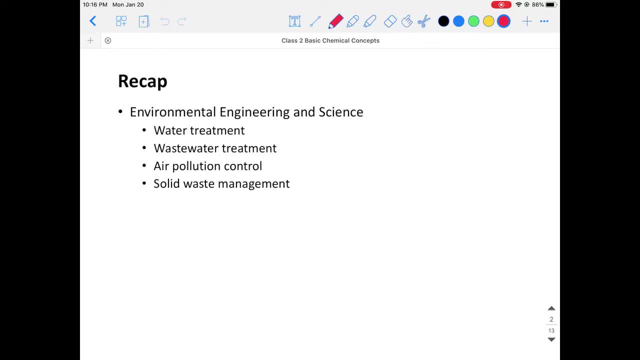 especially in the water treatment, wastewater treatment, air pollution control and solid waste management right. So as we further go into this class, we're going to learn more Contents regarding how each system works and how we can design an appropriate system to mitigate these problems. 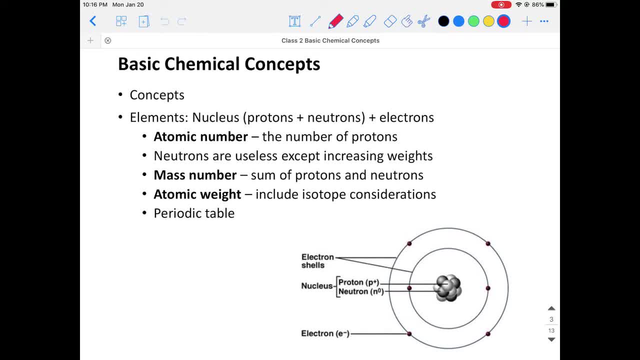 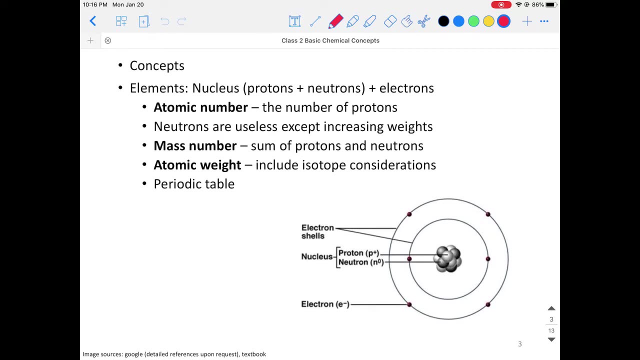 Okay so for this class, as I said, we're going to review some basic chemical contents. Okay, so we're going to go through some concepts here. So first is on the elements. Okay so, as we know from the physics, that the elements is composed of nucleotides. 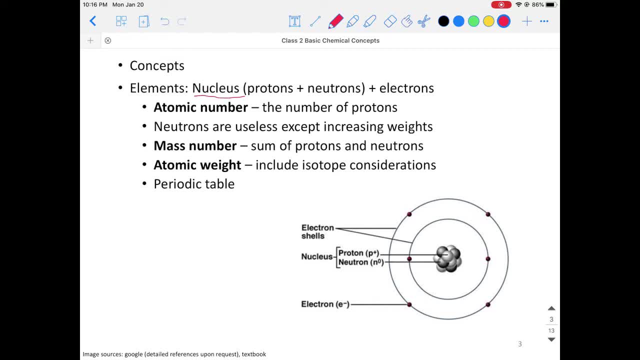 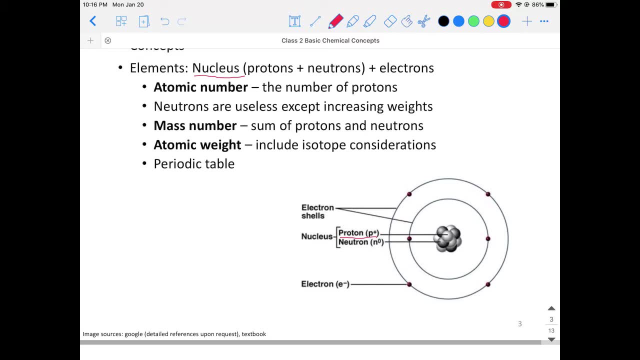 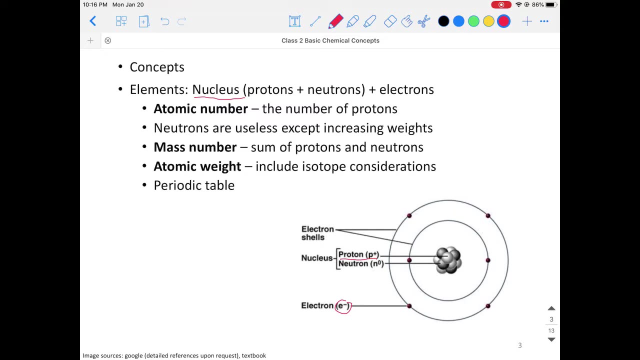 Nucleus and electrons. Okay, and further, the nucleus is composed of protons and neutrons. So basically the protons will carry positive charges and the electrons carry negative charges, And typically for an element the total charge is zero. right. 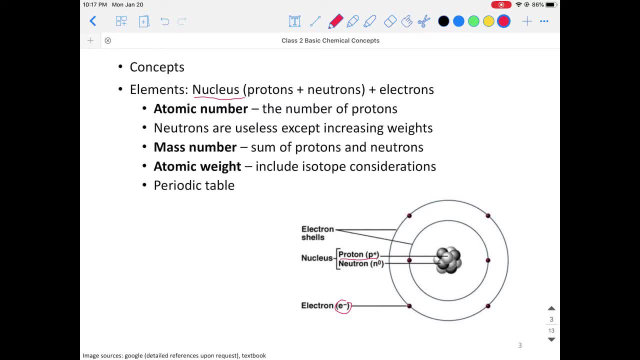 It means that it's neutral. So that's why the number of protons are going to be equal to the number of electrons. for a neutral element And further, the atomic number is basically the number of protons. For example, the hydrogen will have an atomic number of one and the carbon will carry an atomic number of six. 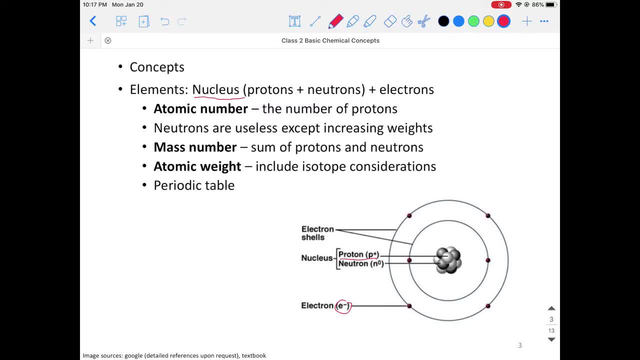 So we can basically say that the neutrons are useless in terms of charge, except increasing the weights, Because for a lot of elements, for example carbon, have many isotopes and for each of these isotopes the atomic number is the same, because that's the reason why we call them as carbon. 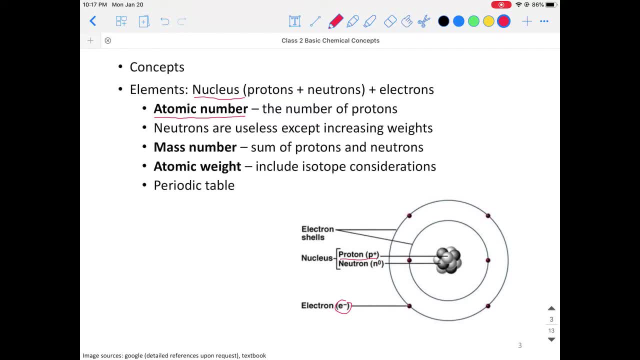 Because the number of protons are the same, that's exactly six, But the number of neutrons are different for different isotopes and that is giving the carbon different, the different isotopes of carbon with different weights, or the mass number. So basically, the mass number is the sum of the protons and the neutrons. 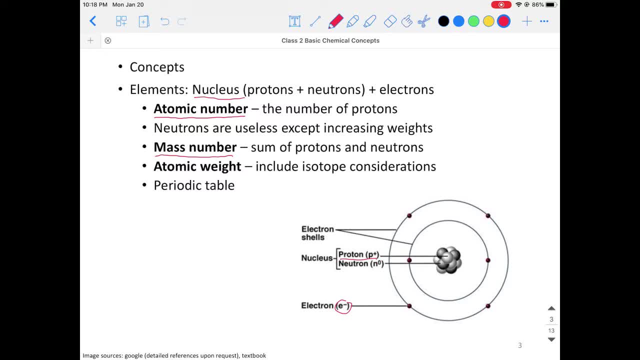 So basically it's the number of protons and the neutrons. So if we add up the number of protons and add up the number of neutrons, and that's going to be its mass number. And, furthermore, when we talk about the atomic weight, we're not talking about the mass number. 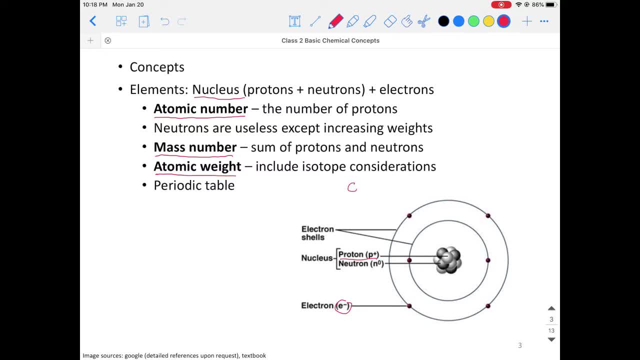 but we're considering different isotopes, For example carbon. you have a certain amount of carbon- 12- and you also have a certain amount of carbon 13.. So you notice that here I write the number of protons and the neutrons. 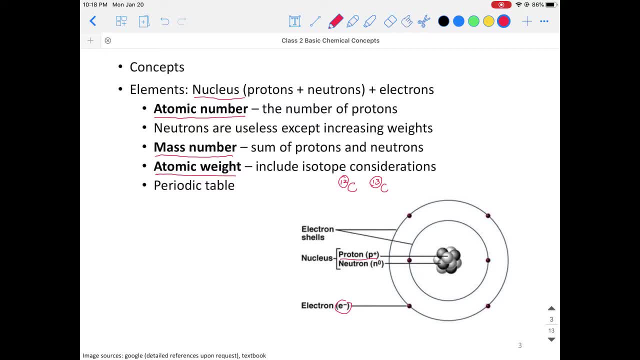 And you sort of specify the number of neutrons here in the left top corner and then you sort of define the mass number on the left top corner, which means that this is the number of protons And this is the number of neutrons. 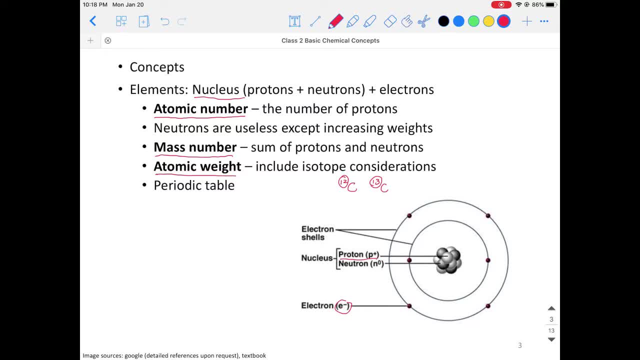 And, as we know, the number of protons for these carbons are exactly the same. right, they're 6.. This means that carbon 12 has six neutrons, While carbon 13 has seven neutrons. okay, So with this fundamental information on the elements. 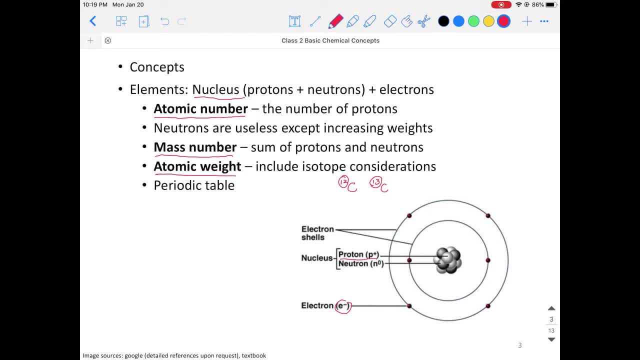 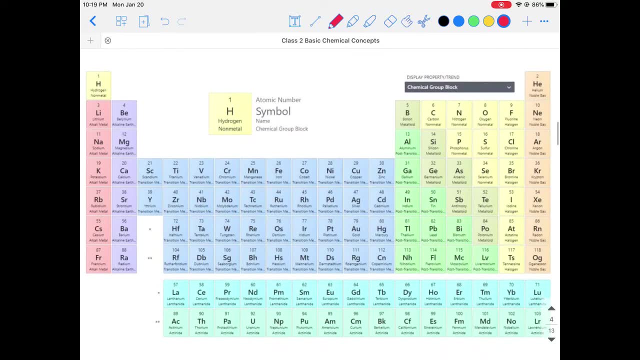 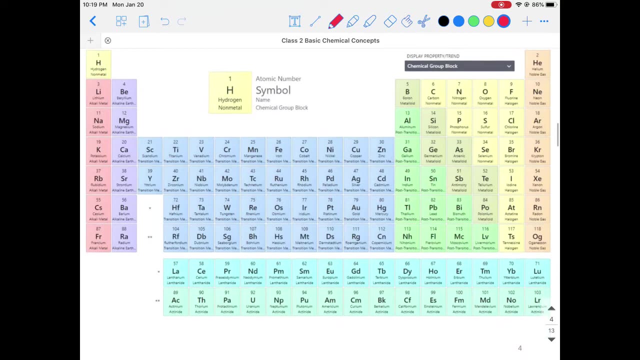 know we can basically rank them onto a table here based on its, based on their atomic number, and that is giving us the periodic table. so here in the periodic table you can see that along each row here the atomic number increases. it starts from one to the end of 103, and we should notice that. 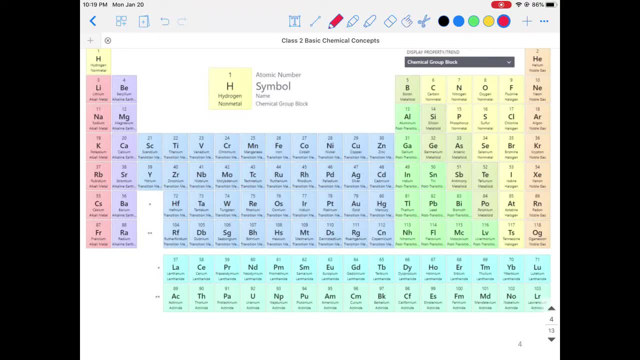 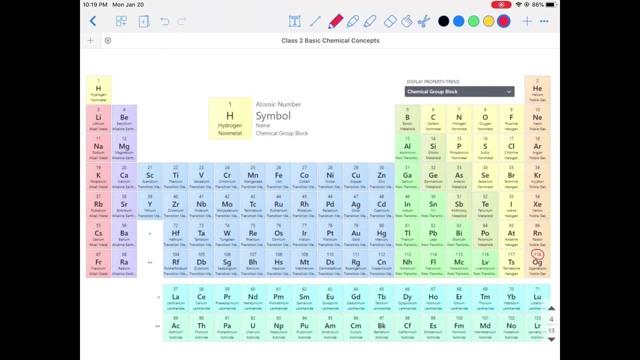 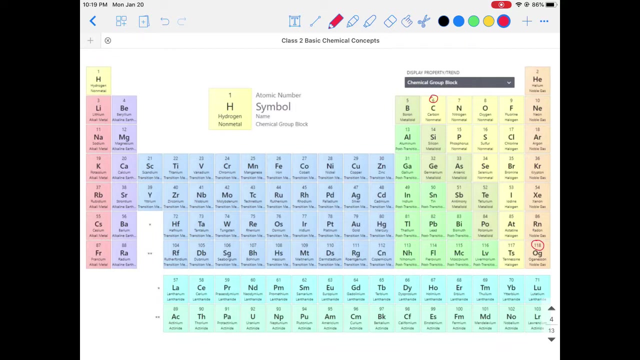 there are a lot also. there can be further more elements, it's just that they are not stable enough. actually it's 118, okay, on the bottom right corner here, so you can see that, as I said, the carbon has six protons and that's why it has an atomic number of six. for oxygen, it has an atomic 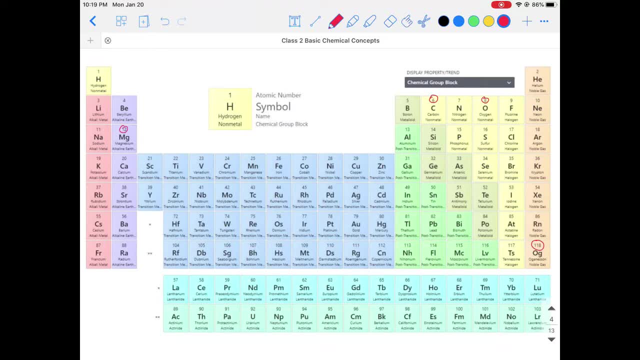 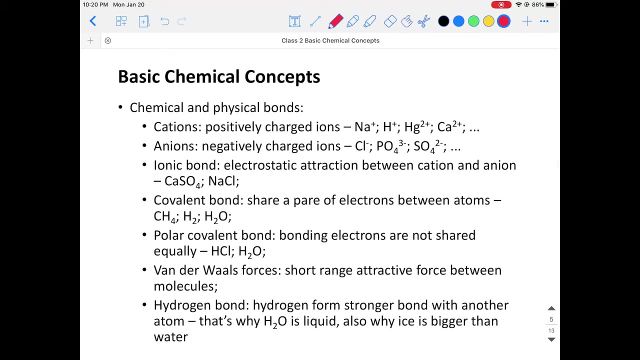 number of eight. right for magnesium, you have an atomic number of 12. okay, so this is how we can find each other, our, if each of our, elements on this periodic table, And after we know the elements, we can start to know what are the interactions between the elements when 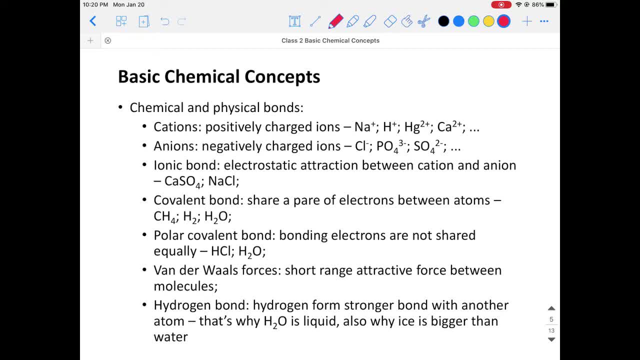 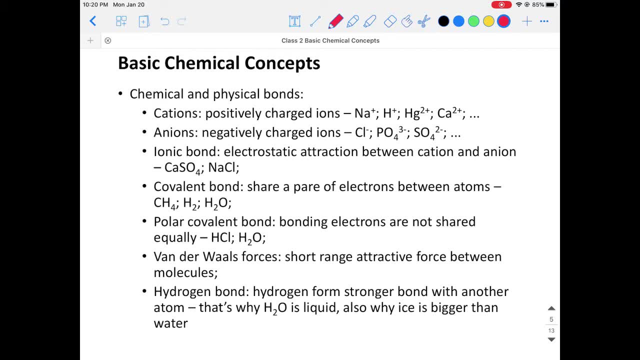 we're forming different types of compounds there, So there are different types of physical and chemical bonds, For example for the elements. we can further differentiate them, or, if they carry certain charges, we can name them as cations or anions. The cations are basically positively charged ions, For 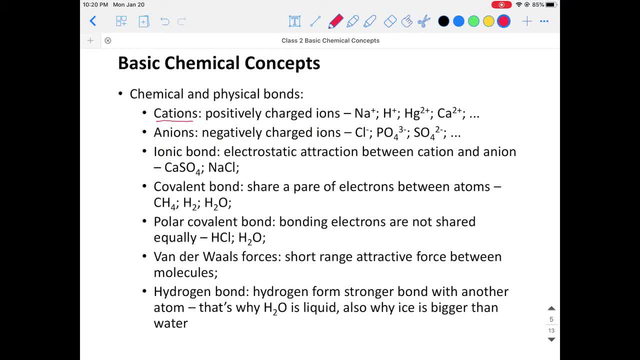 example, the sodium ion, the hydrogen ion, mercury ion, calcium ion. So they will carry positive charges, which is because they lost their electrons. So that is giving them because we are losing negative ions, and that is giving them a positive charge And in terms of the anions, basically we are. 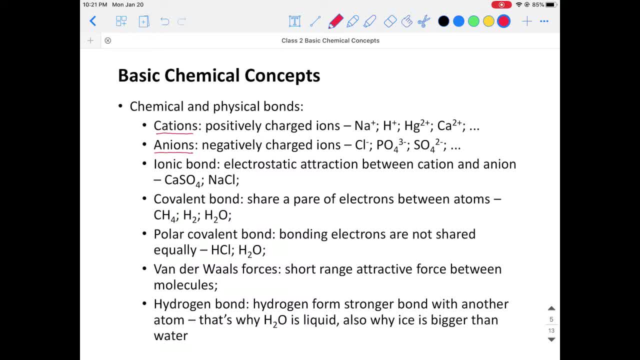 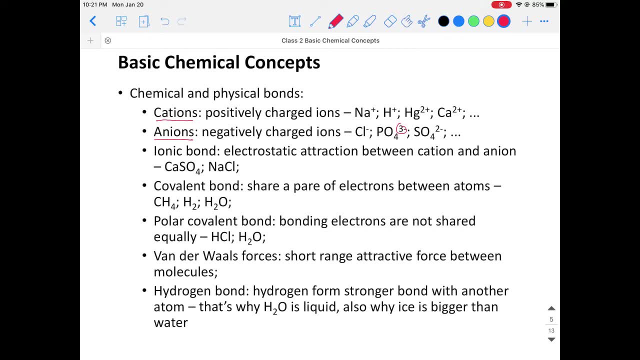 adding more electrons onto these elements, For example the chloride ion, the phosphate ion and the sulfate ion, And you notice that there are different numbers here, right? This basically means that how many extra? what is the difference between the number of elements for these ions? 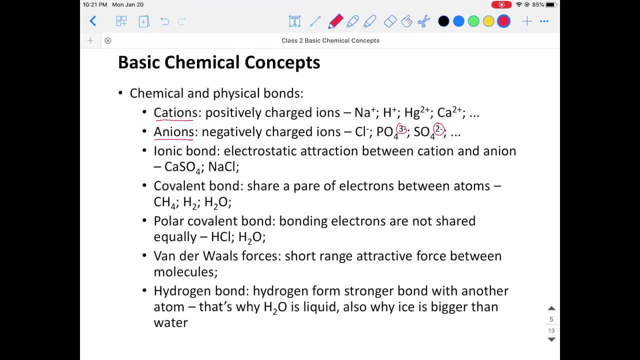 compared to the original state or the neutral compounds. For example, the phosphate ion carries three extra electrons and that is giving it a negative three charge right, And on the other hand, for the calcium ion, basically it lost two electrons and that is giving it a positive two. 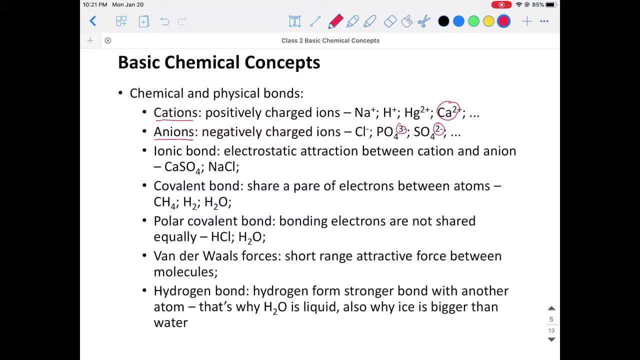 charge And after we have these ions, and basically these ions can form ionic bond. For example, the calcium can compound with the sulfate and the relationship or the bound bonding between these two parts or these two ions is called ionic bond. So basically that is the electrostatic attraction between the 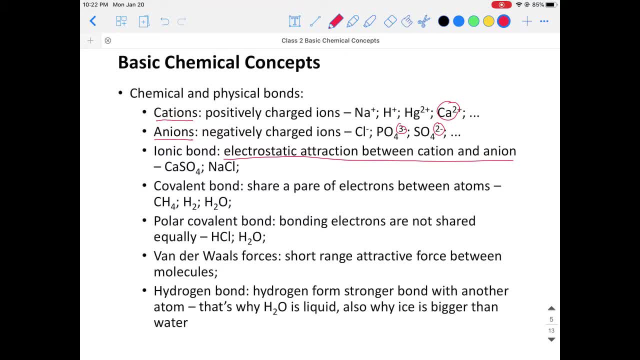 cation and anion, For example the calcium sulfate and the sodium chloride, right. So we can also form ionic bond between these two elements And on the other hand, in contrast, there are also covalent bonds, which means that, basically, 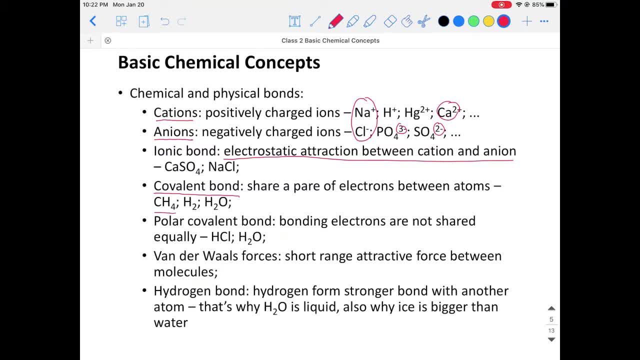 these different elements that are formed within this compound. they were not ions in the beginning. For example, the methane here. So basically we're not saying that the carbon here has a negative four charge, Or the hydrogen here has positive one charge. So basically they were not ions in the beginning. 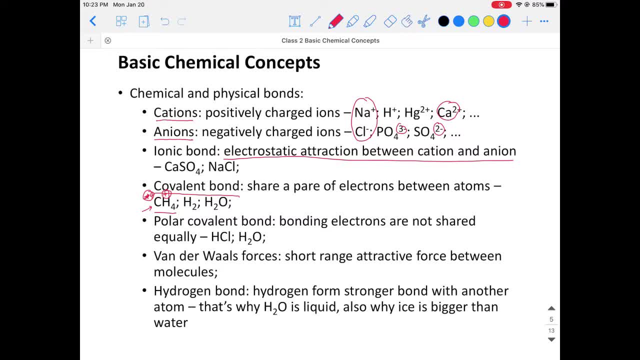 And what happens is that these elements will share their electrons instead of giving up or accepting electrons from each other, And that is why the covalent bonds describes a share of a pair of electrons between the atoms. okay, So this also happens for a lot of the gas species, For example. 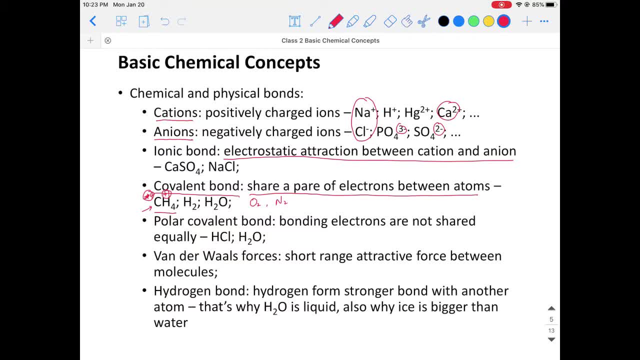 the hydrogen right, And also oxygen, nitrogen, so on and so forth. So basically, for in these species the elements are sharing their electrons instead of giving up electrons from one side to the other side, And this also happens for water here. So the hydrogen and oxygen also sharing their electrons. 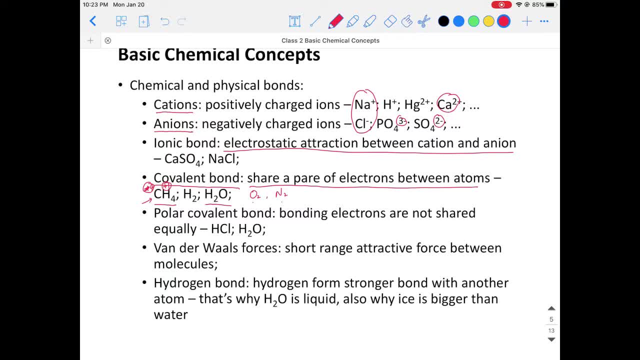 But we should notice that even though they're sharing the electrons, even though they're shared, they're not shared equally, For example, in terms of the oxygen, in terms of the water here. So, basically, because the oxygen is more needy of the electrons. so the shared electrons between the 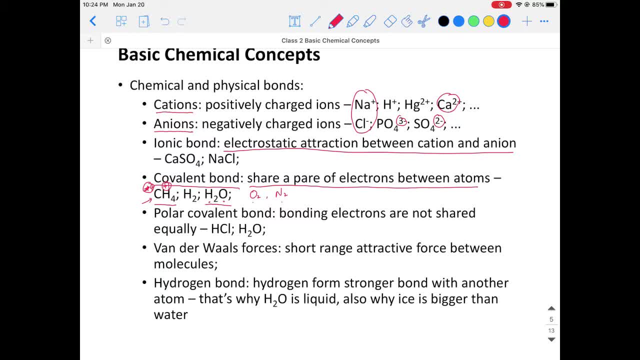 hydrogen and the oxygen will move more closer to the oxygen here, right? So because of this, we're going to form these polar covalent bonds. So we're going to form these polar covalent bonds. So, basically, these electrons are not shared equally between the elements. So, as I said, 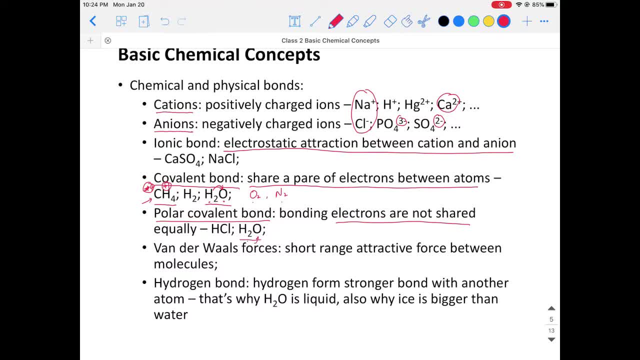 for water, the electrons would tend to get closer to the oxygen and get farther away from the hydrogen here, And the same also applies for the hydrogen chloride. So the electrons from the hydrogen will stay closer to the chloride, well further away from the hydrogen. 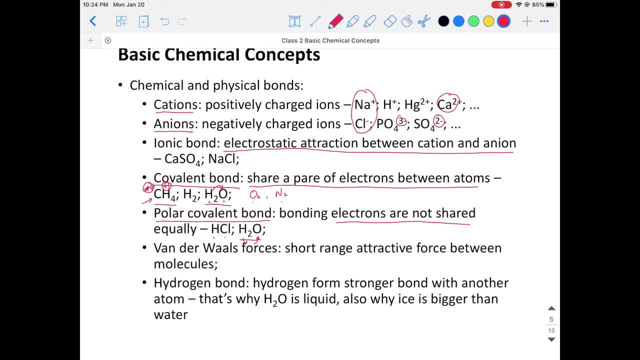 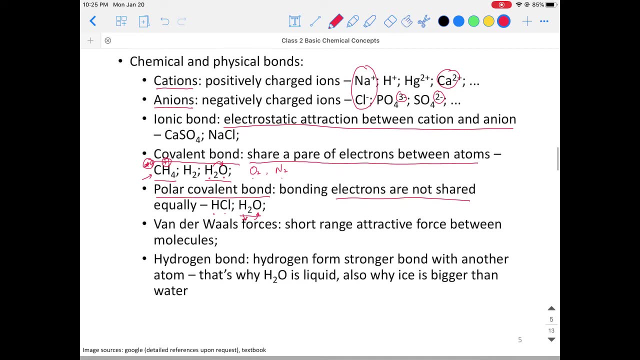 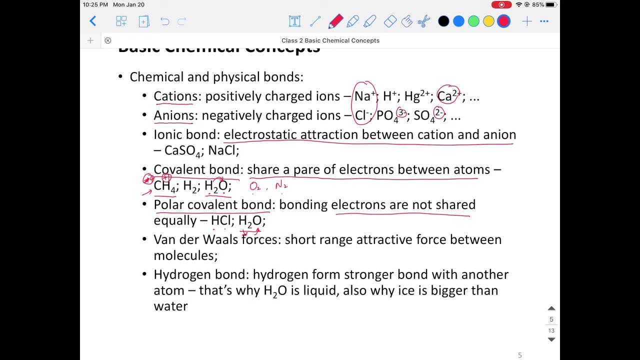 but these two elements are not forming ions. For example the hydrogen here in hydrogen chloride. it's not a cation, while the chloride is not an ion. So after these interactions there are also van der Waals forces and this is actually a physical bond between different. 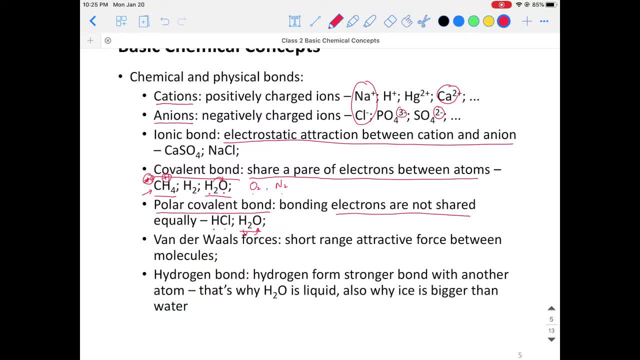 species. So the van der Waals force is a short-range attractive force between the molecules. So, as you can see, when we talk about the bondings here, we're talking about the. when we talk about the bondings here, we're talking about the interactions between the elements. 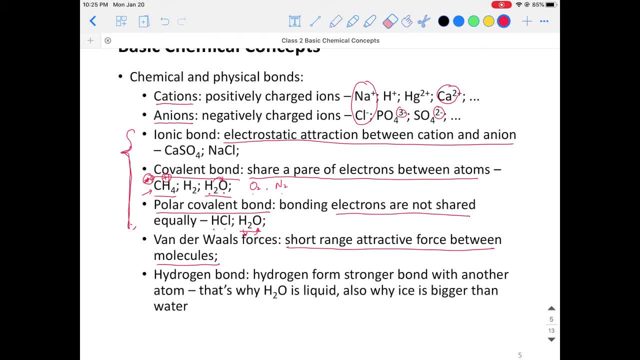 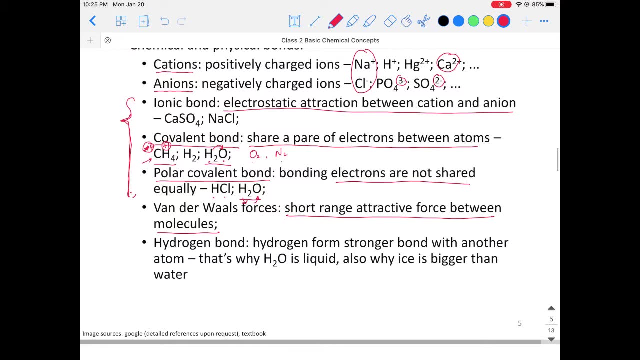 that's within the compound. but the van der Waals force is talking about the interactions among or between the molecules And that is why it's not a prerequisite for the compound. And there is also hydrogen bond. So basically, the hydrogen bond means that let's say, here's our water molecule. 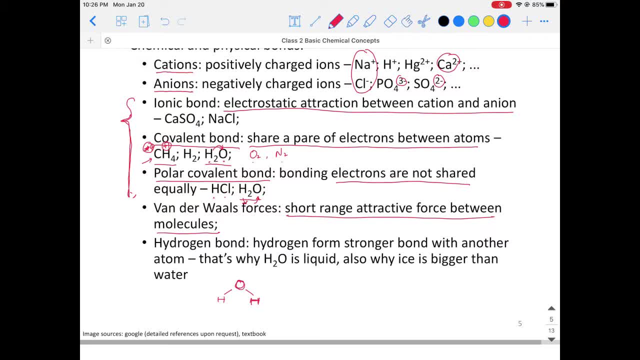 So because the oxygen is more needy of the electrons, so it also tries to bond with other hydrogens. So it's basically forming a weaker interaction between molecules And because of this hydrogen bond, the water is in the liquid phase under the normal conditions And this is also why the ice 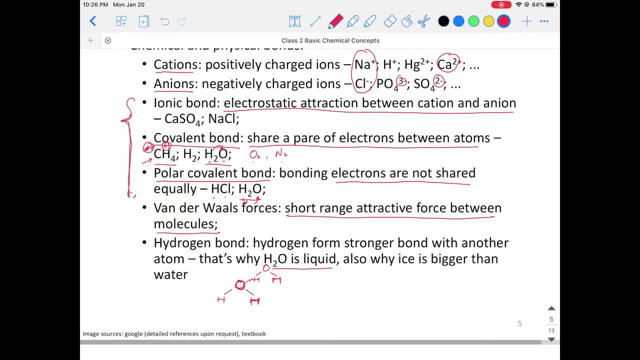 which is a frozen or a solid state of water, is bigger than water. That is because during the water, during the liquid state, there are easier hydrogen bonding between all the different molecules. So there's a larger interaction between different or among all the different water molecules. 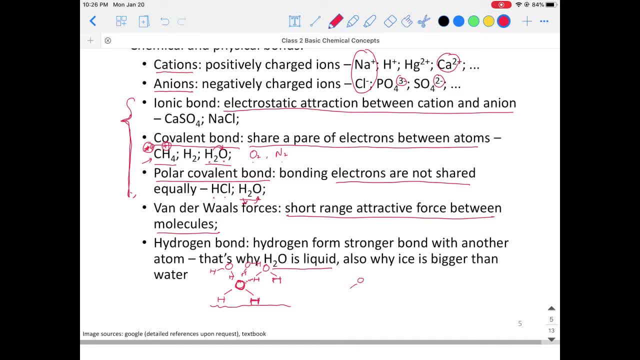 they can arrange in a random state, But once it's frozen it's going to form a more patent interactions And this is going to give us a larger volume of the water and there is solid state, all right. so this is about the interactions where the chemical or 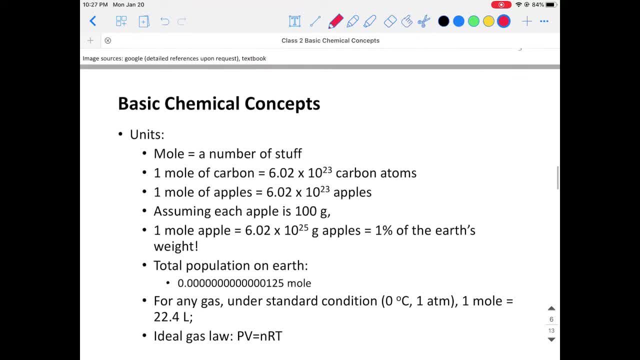 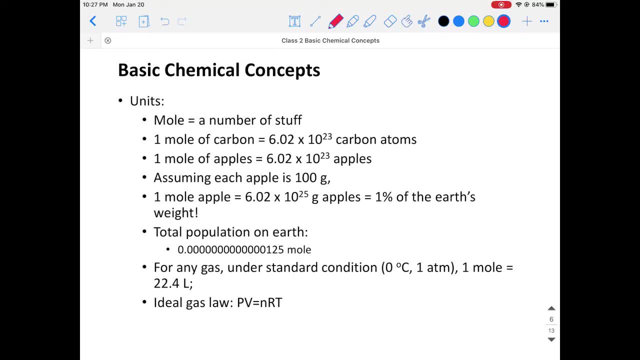 physical bonds between the elements and also between the molecules. and then we can talk about the units. okay, the most widely unit in the environmental engineering is the mole. okay, so basically the mole represents a number of stuff. it can be a number of any stuff. for example, if we say that there's one, 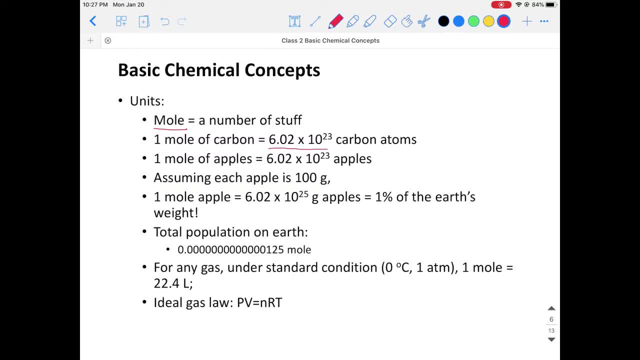 mole of carbon, then that means that there is 6.02 multiplied by 10 to the 23rd number of carbon atoms, and we call this special number as the Avogadro number. okay, so we can use this mole to describe anything. for example, we can say that: 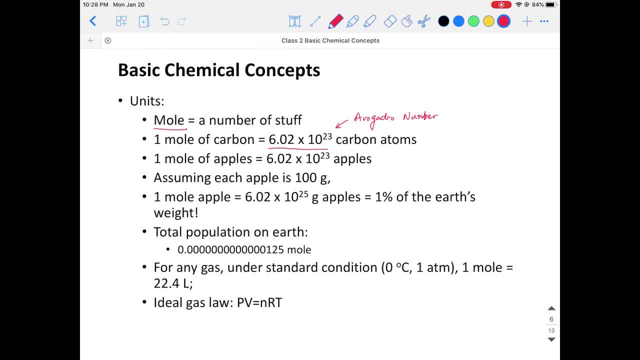 there is a mole of F. okay, so we can use this mole to describe anything. for example, we can say that there is a mole of F- apples, and that purely means that there are 6.02 multiplied by 10 to the 23rd number of apples. so further, let's say, let's get an understanding, what is the? 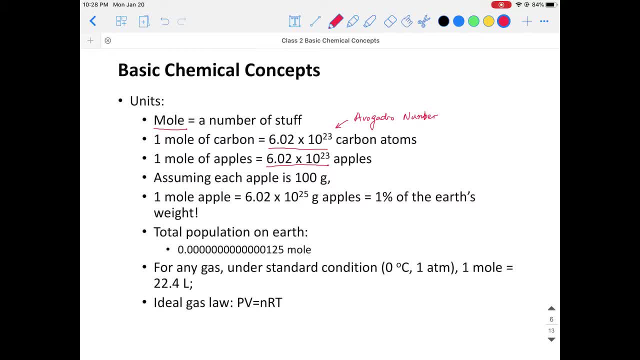 magnitude of this Avogadro number. so basically, if we assume that each apple is 100 gram and then one mole of apple is going to be 6.02 multiplied by 10 to the 25th gram grams of apple, which is already around 1% of the earth weight. so you can see how large this number is. so also, 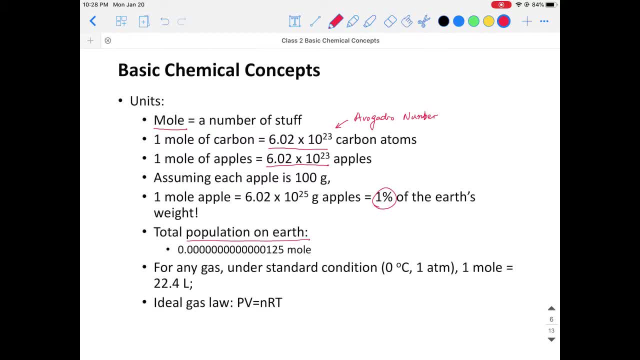 let's consider the population on the earth. so we know that the population on the earth is what? around 7 billion on the on the earth. right, that's quite a considerable or a significant number, but if we try to consider this number in moles, so you can see that there is almost a. 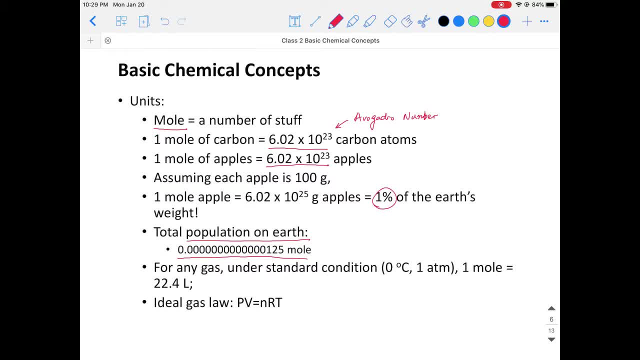 uncountable zeros there. so we're still far away from one mole of people on the earth. right, and you can also see that if there's really one mole of people, how large of a crowd that is going to be right, so you can see that the mole is a. 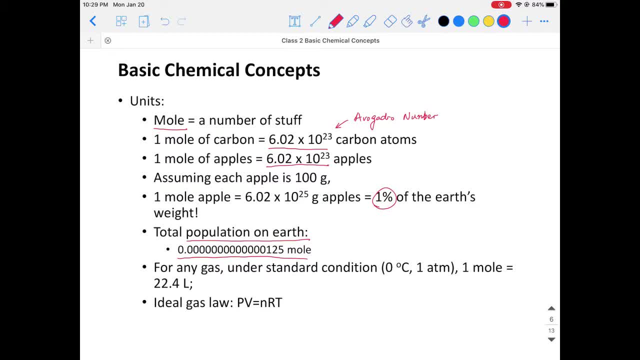 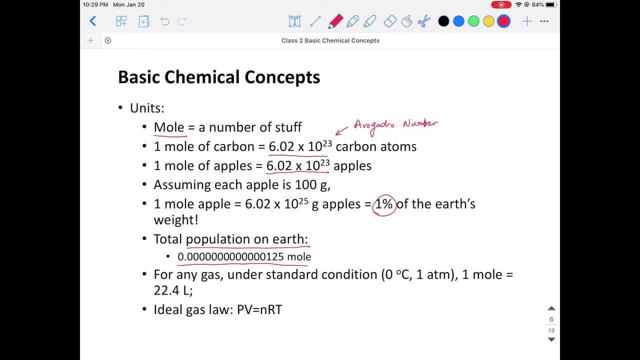 very Avogadro number. it's a very large number that we can use to describe the amount of atoms, and this is indeed the case, right? so, for example, we know that the molecular weight or the mass number of water is 18, right, It represents 18. 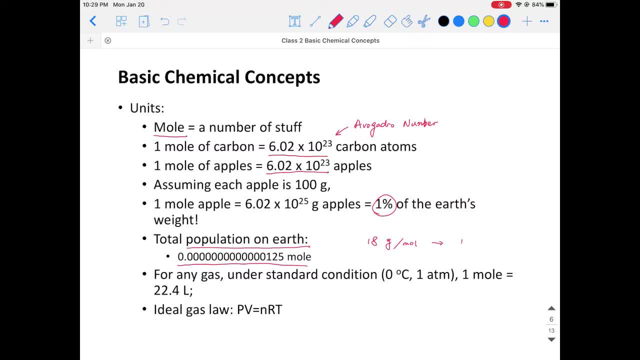 grams per mole. So basically that means that if we have 18 grams of water, then that's going to be exactly 6.02 multiplied by 10 to the 23 number of water molecules there. So you can see that there is really a large amount of 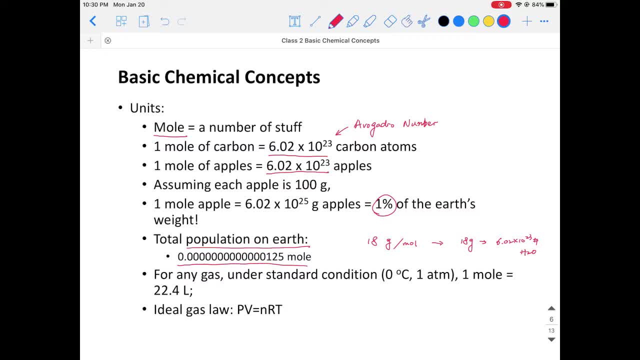 these molecules in in this state And also from this process you can see how small a molecule is. right, Because 18 grams of water is just 18 centimeters of water under normal condition and 18 centimeters is not a lot. So you can see. 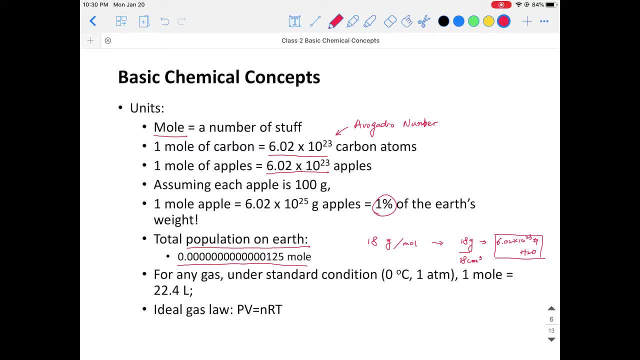 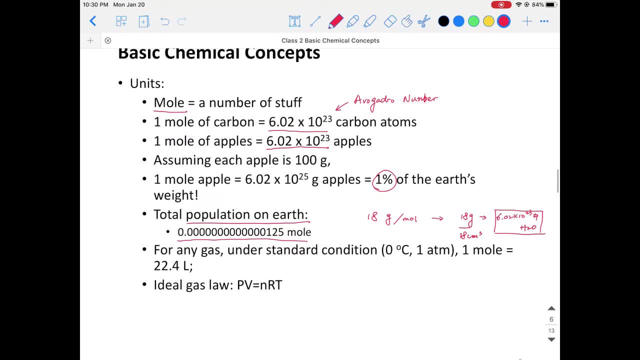 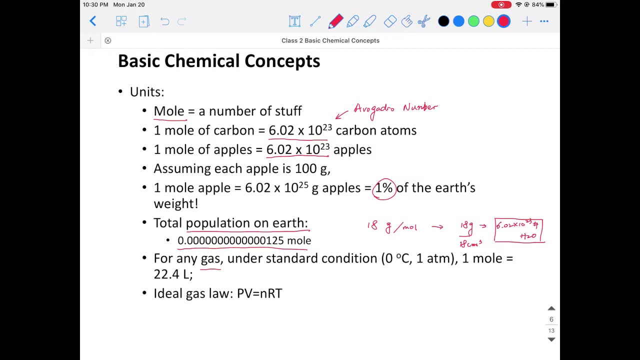 that also, the size or the volume of the water is also very significantly small. okay, And also for any gas or for any species that's in the gas state under the standard condition, which means that it's zero Celsius and under one atmosphere. so 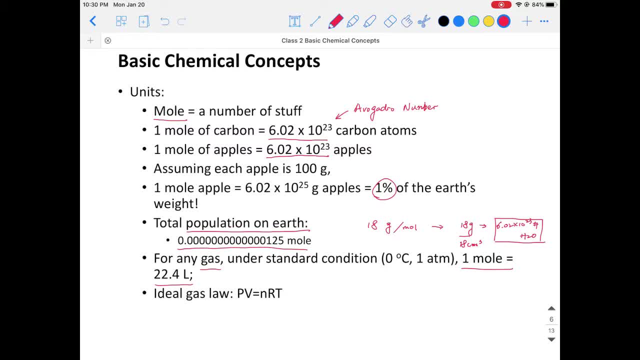 one mole of this gas species is exactly 22.4 liters. So this applies for any type of gas species, no matter it's oxygen, nitrogen, ammonium, so on and so forth. So the reason why the volume is always a constant: always 24.2 under this standard. 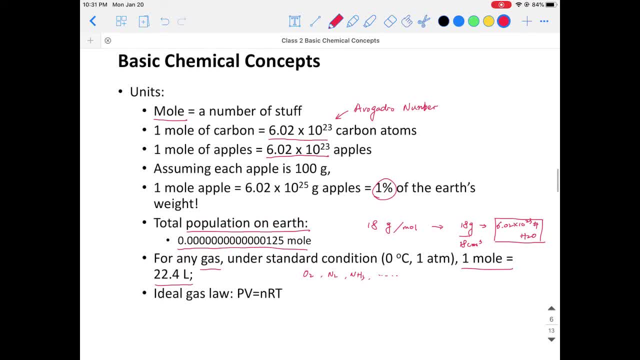 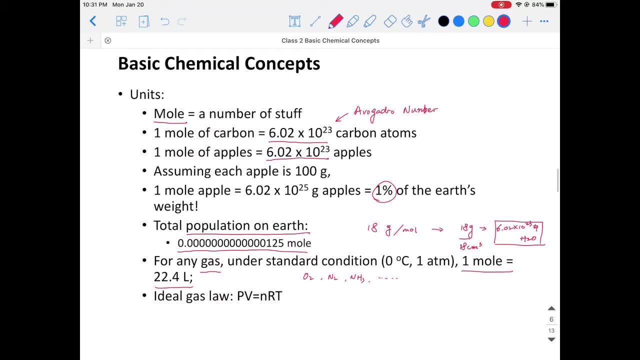 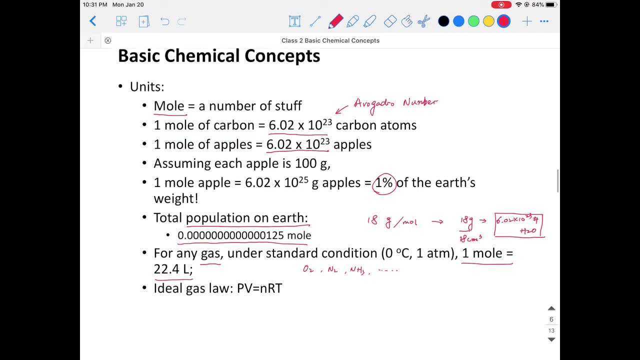 condition is because of the ideal gas law. So basically, ideal gas law represents or describes a physical state of any gas species. I know that some of you also prefer to call that as a PefNert right. PV equal to nRT. Okay, And we also. 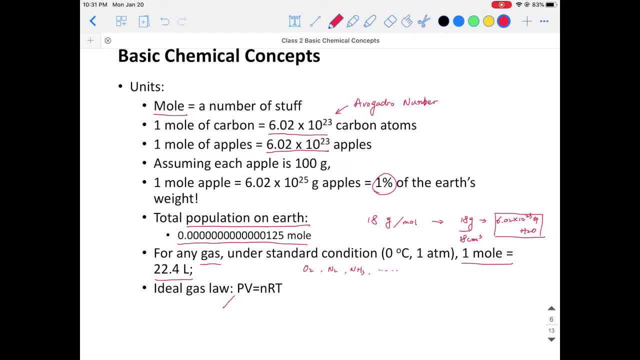 pay attention to the units of this ideal gas law here. so basically the p here will carry a unit of pascal, okay, b here and carry a unit of the meter cube, right. so n carry a unit of mole t here carry a unit of kelvin, okay, so basically the temperature in kelvin. 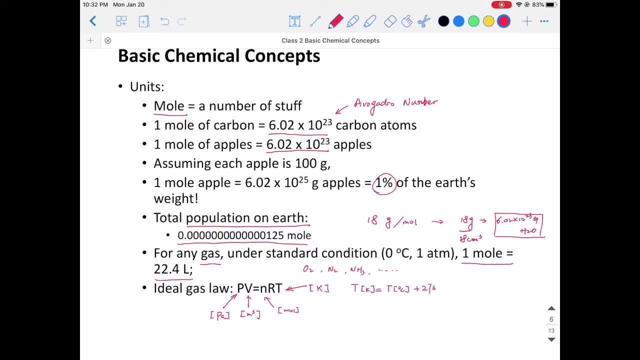 is equal to the temperature in celsius plus 273.15 kelvin. okay so, and only under this condition, and only under these units, the r here will have a value of 8.314 per mole. okay, so, it's only joule per mole per k. 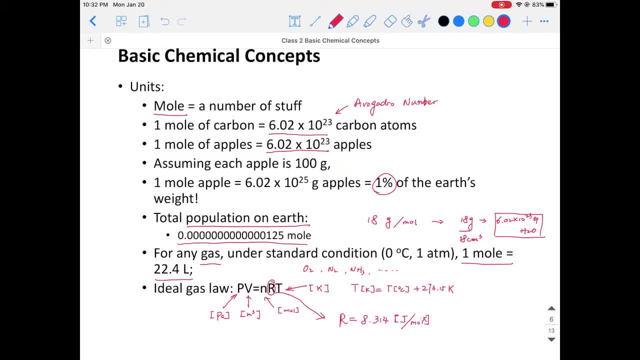 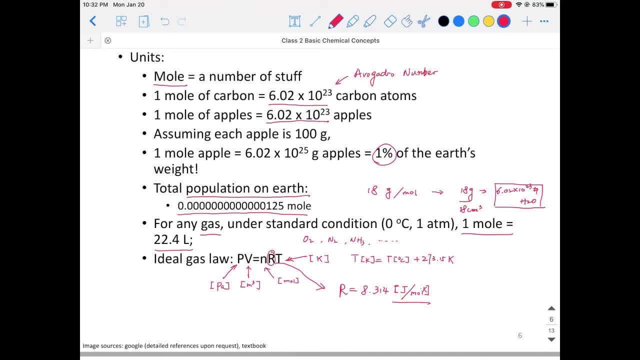 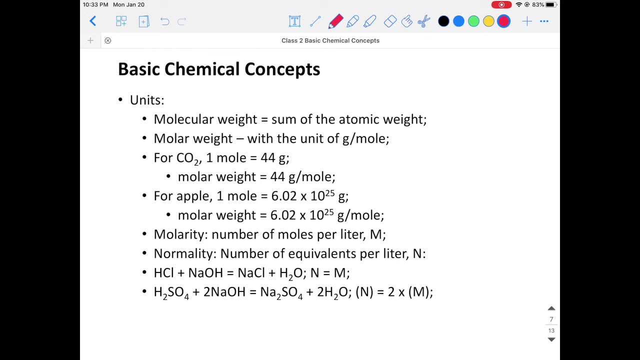 so it's only under this condition that we're going to have this specific value of the gas constant and also have this unit here. okay, so further, as i said, there is a concept of the molecular weight. so basically, the molecular weight equals to the sum of all the atomic weight. for example, we give: 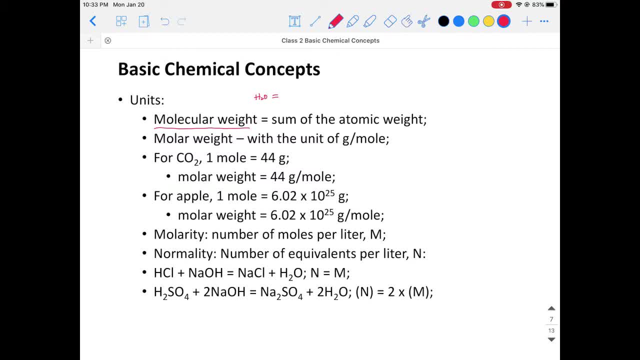 the case for water. so for water, the atomic weight is going to be, or the sum of the atomic weight is going to be, 2 multiplied by 1 plus 16, right? we're talking about the atomic weight, not the atomic number, right? so that is going to be equal to 18 gram per mole. 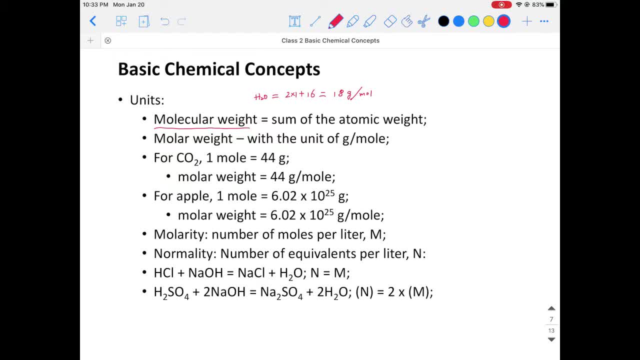 so this is the unit of the molecular weight. okay, for carbon, one mole of carbon. for one, one mole of carbon dioxide. let's try to calculate again. molecular weight of carbon dioxide is equal to the molecular weight of carbon, which is 12 plus there are two oxygens: 2 multiplied by 16. 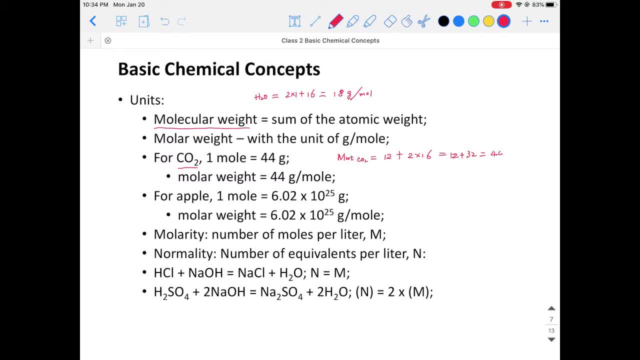 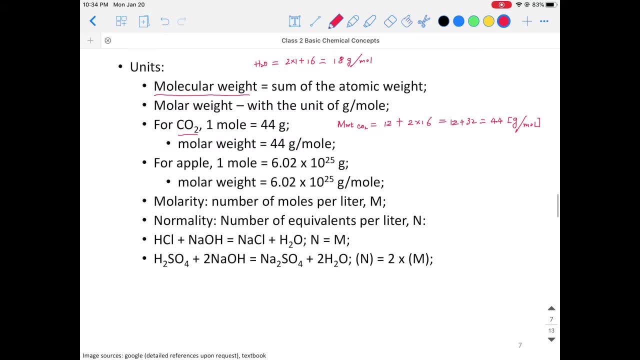 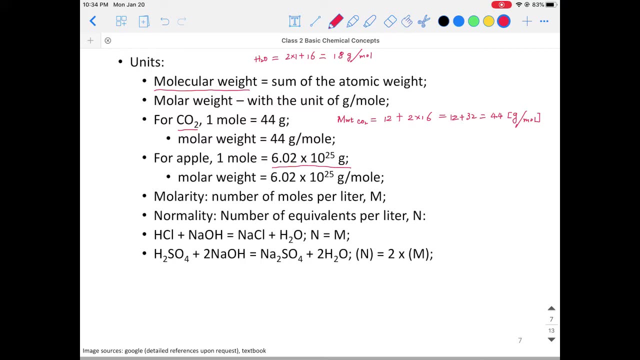 it's going to be 12 plus 32, which is equal to 44, and it's going to carry the unit of unit of gram per mole. okay, so we know that for Apple here, one mole of Apple is equal to 6.02 multiplied by 10. 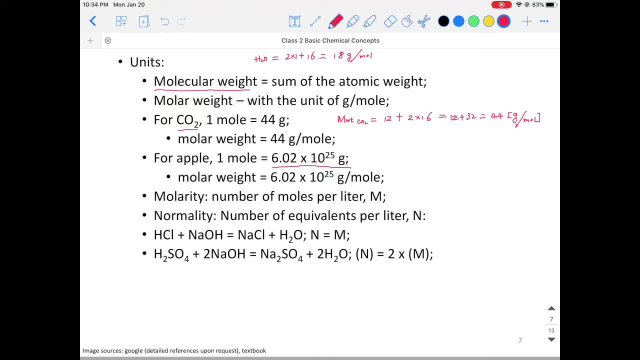 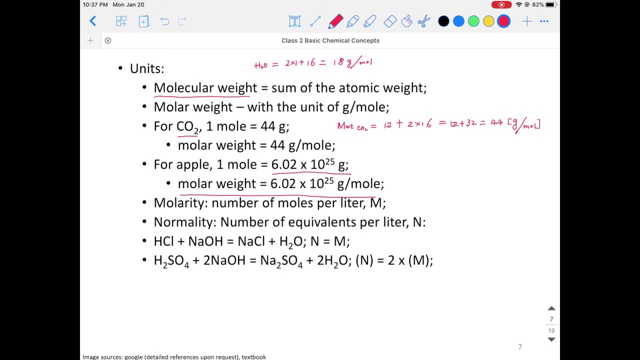 to the 25 grams. so for that reason we can tell that the molecular weight of Apple it's going to be this large. this is really a significant amount of mass there and furthermore we have the definition of the molarity. so the molarity means for a solution. for example, we prepared some solution. 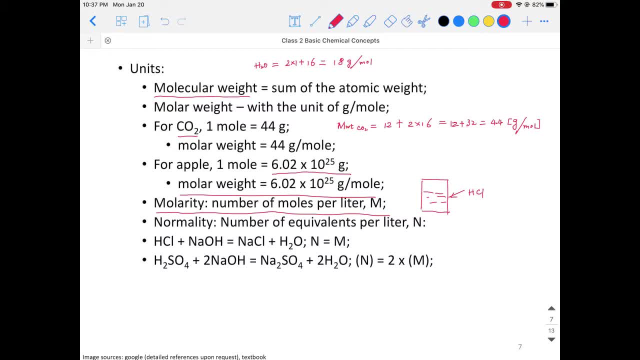 there, and let's assume that this is hydrogen chloride. so what is the number of moles per liter, for example? let's assume that the the volume of this solution exactly one liter there are. so then the molarity means that how many moles of hydrogen chloride are there in this solution? 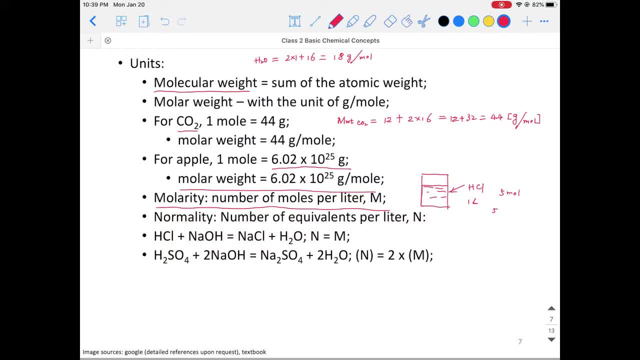 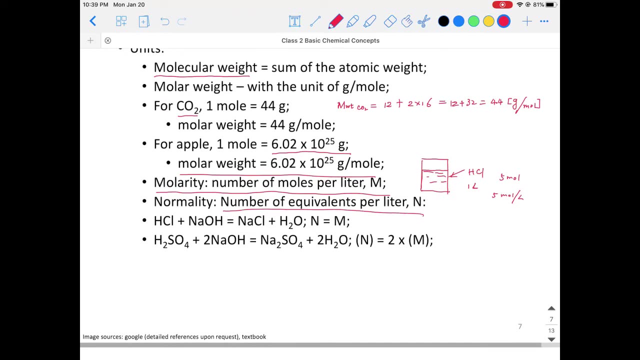 for example, if there are five moles, then the molarity is going to be five mole per liter, right? similarly, we can have the definition of the normality. so the normality is defined as the number of equivalents per liter, and this applies when we're trying to solve or when we're 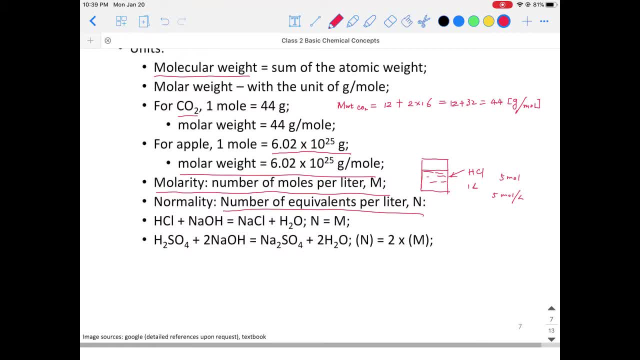 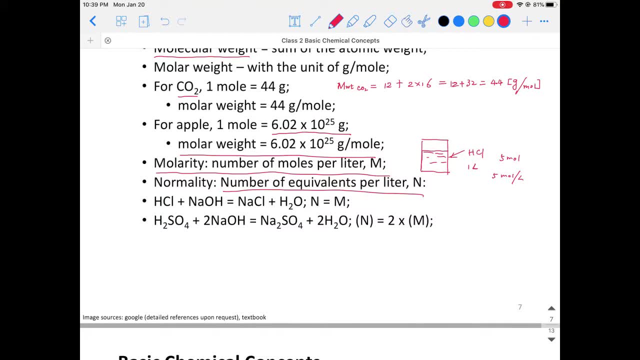 to study the ions with more complex structures. For example, here let's consider the neutralization of the hydrogen chloride and sodium hydroxide, Because both of these chemicals have a very simple structure there. so there's going to be a one-to-one ratio here and that is going to 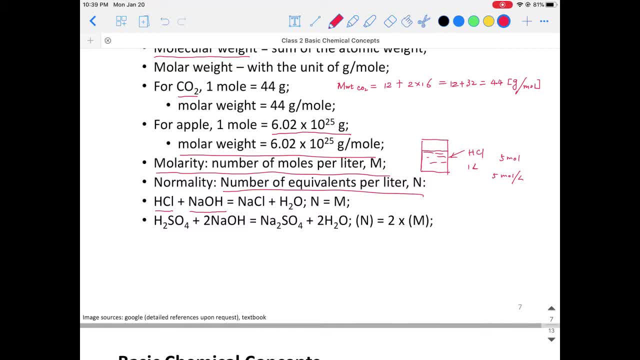 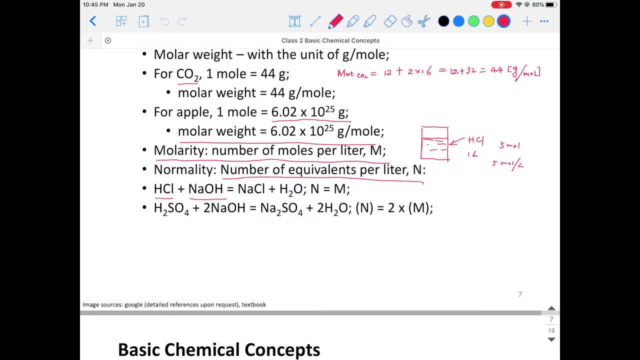 give us a result that the normality is equal to molarity. And for a system that's containing the sulfuric acid and sodium hydroxide, the normality and molarity are going to have different relationships, because right now we need two moles of sodium. 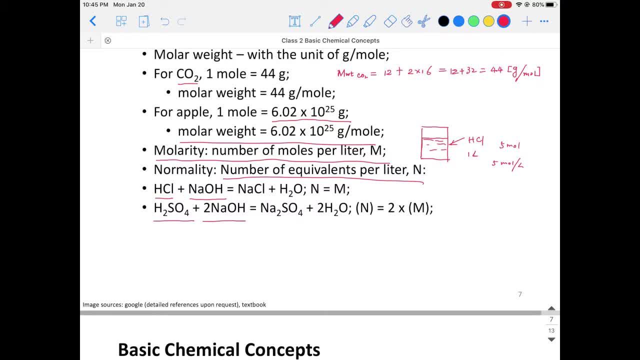 hydroxide to neutralize one mole of the sulfuric acid, and this is the reason why the normality of sodium hydroxide is equal to molarity. The normality of the sodium hydroxide is going to be two times of the molarity. 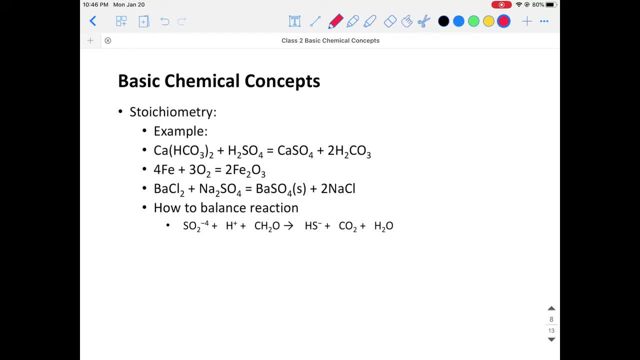 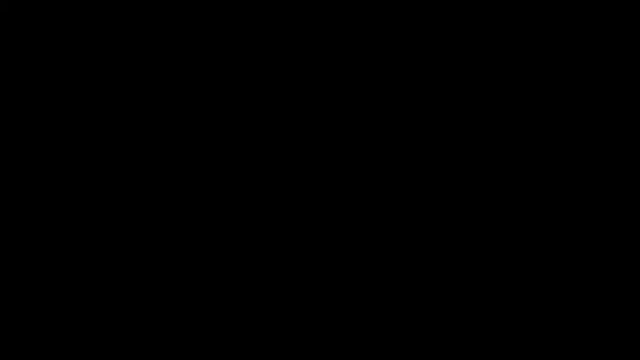 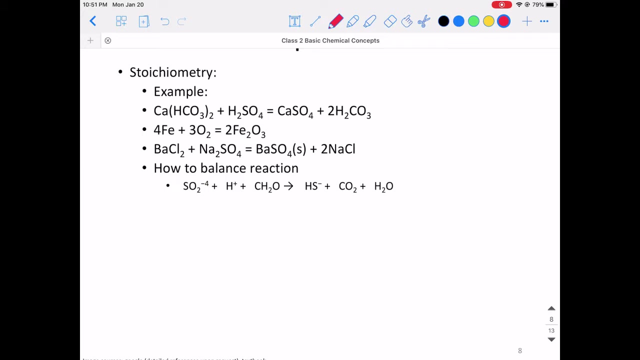 And furthermore it's the stoichiometry. So stoichiometry means the complete reaction of all of the reactants. So basically, if we write out the chemical reactions, there is no net gaining or net losing of any elements. So, for example, if we're trying to balance the equation or balance the reaction between the 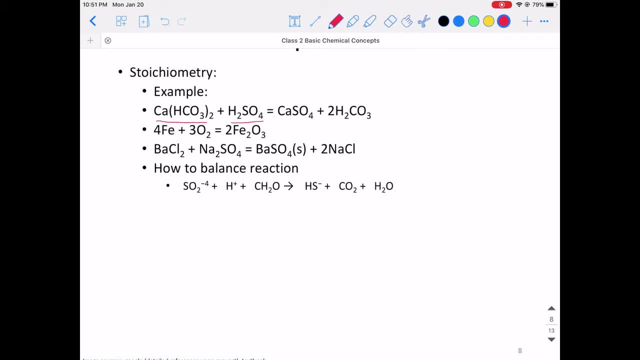 calcium bicarbonate and sulfuric acid. we know that the calcium and sulfate ion are going to have a one-to-one ratio and that is going to form the calcium sulfate right And at the same time the hydrogen here are going to react with the 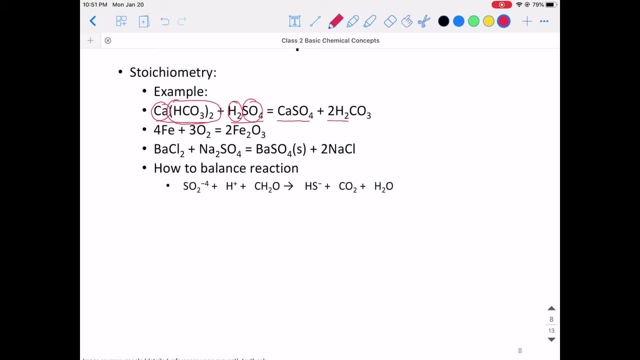 bicarbonate ions here, And that is going to give us two numbers of the carbonic acid, right? So this is the reason why the numbers in front of the first three compounds are one, and then we're forming, basically forming two moles or two numbers of the carbonic acid. 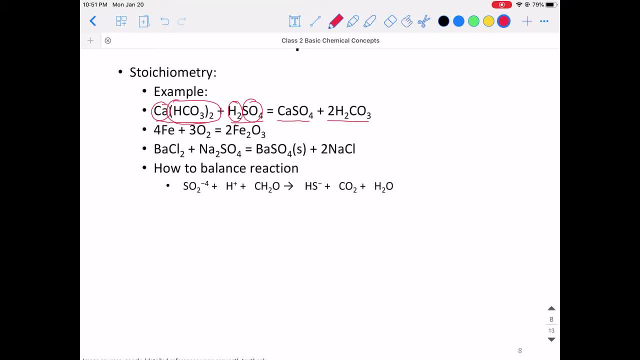 And similarly we can take a look at the reaction between iron and oxygen. So if the reaction is forming iron oxide or sodium sulfate, then the reaction between iron and oxygen is two moles or the ferric oxide. We know that for the ferric oxide the iron here will carry a charge of plus. 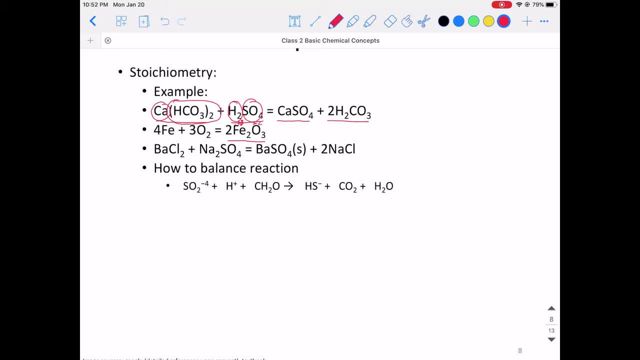 three, right, And at the same time the oxygen here are going to carry a charge of minus two. Okay, so then we need to consider what is the balance on the electrons here. So basically, if we write out the equation on the right hand side here: 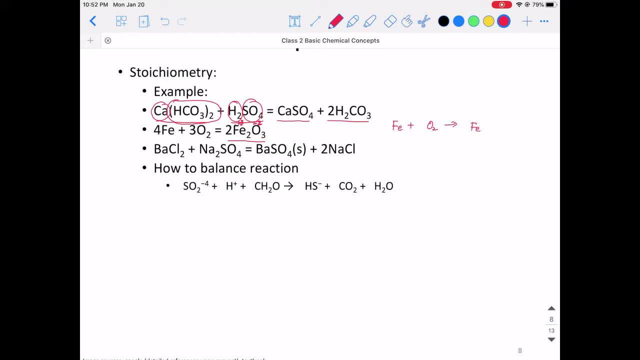 so the iron are reacting with oxygen to form the ferric oxide, right. So on this side we know that the irons here are carrying plus three charge, oxygen carrying two charges. Okay. so that is the reason, because the iron oxide have to be neutral. 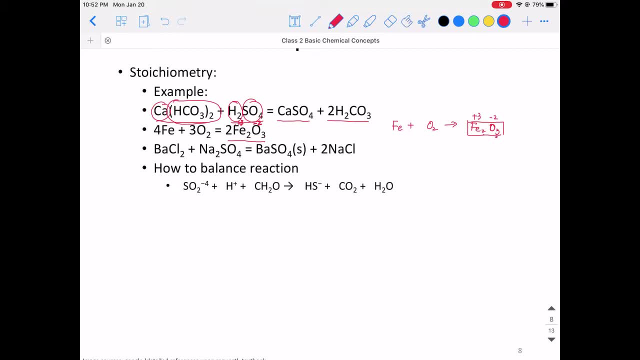 so that this is giving us two numbers of iron and three numbers of oxygen here, right And further. we have to consider how to balance the total number of oxygen here, because on the right hand side the number on the oxygen is an odd number, so we need to multiply this by two and this is going to require three. 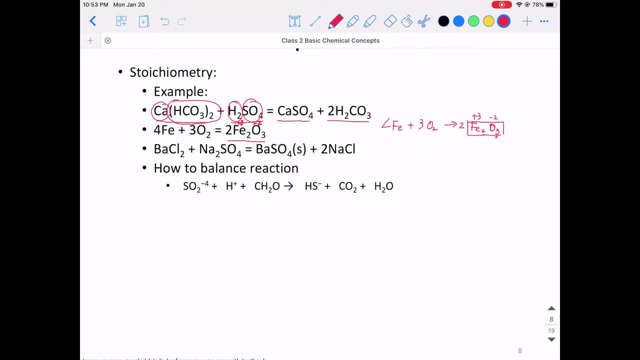 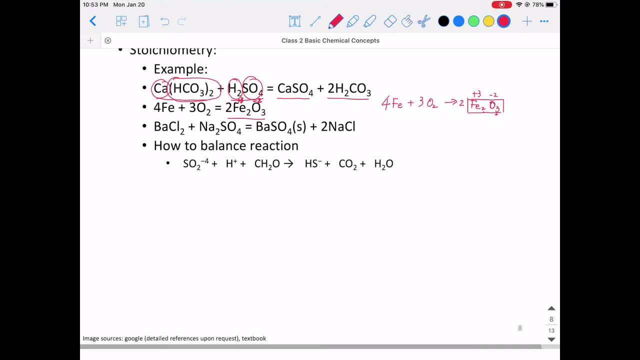 numbers of oxygen. And then if we look at the number of ions, we know that the number of ions are going to be four here. So we can also have a look at the reaction between the barium chloride and sodium sulfate. We know that because the barium have a charge of plus two and sulfate carry a charge of minus two. 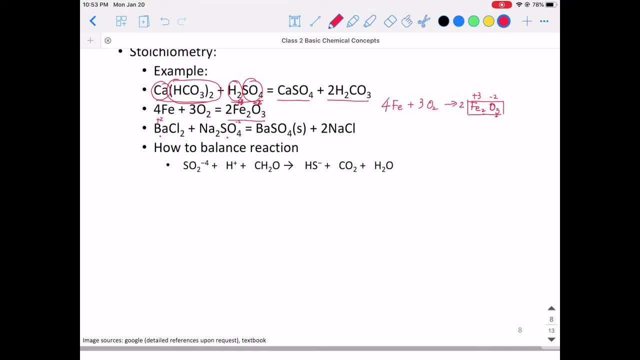 right, So that is going to be a one to one ratio between the barium and the sulfate, and this is indeed giving us one number of barium sulfate. Okay, and then if we look at the sodium chloride, and then that's going to give us two numbers of sodium chloride. So you can see that. 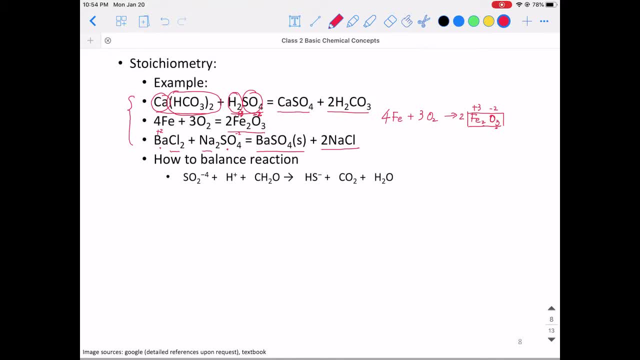 for balancing these three equations. they're quite straightforward, right? It's not taking a lot of efforts, But we have to notice that there are a number of reactions that are not very easy to balance. So let's take this reaction, for example. So, basically, this is the reaction between the 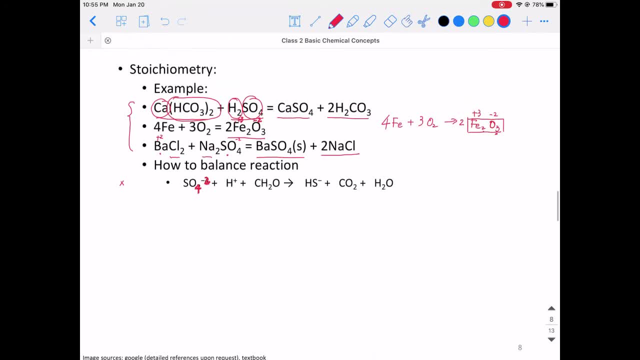 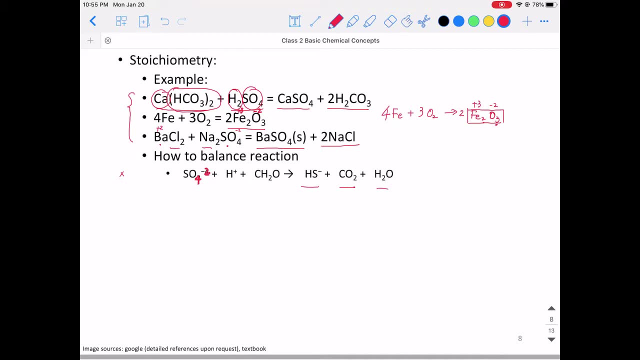 sulfate ion and the formaldihyde, and this is forming a new compound here. okay, Carbon dioxide and water. So you know, to balance this equation here, then it's not very straightforward, right? because we know that here there is a one to one with ratio between the, basically between the. 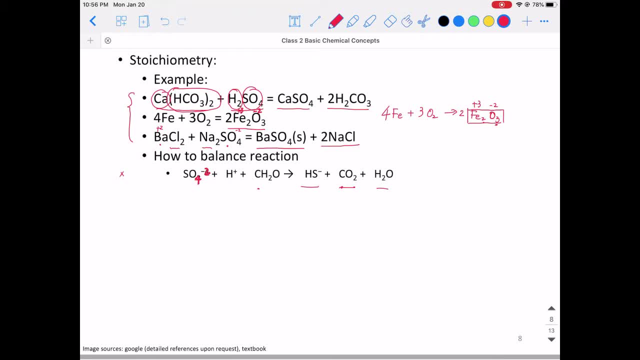 number of carbon left hand side and number of carbon on the right hand side, right. here are all 1 for now, okay, And we also know that the number for the sulfur here should also be corresponding to each other. okay, So we can assume that the numbers here are both a okay. 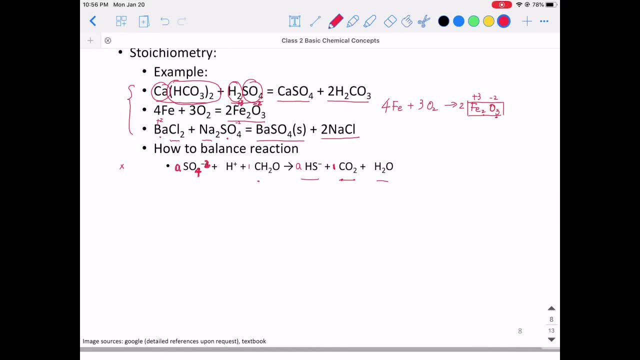 So then let's try to calculate or then let's try to balance this equation, because we need to not only balance all of the elements, we also need to balance the charges. You can see that charge on the left hand side are going to be affected by both the sulfate ion and the hydrogen ion. 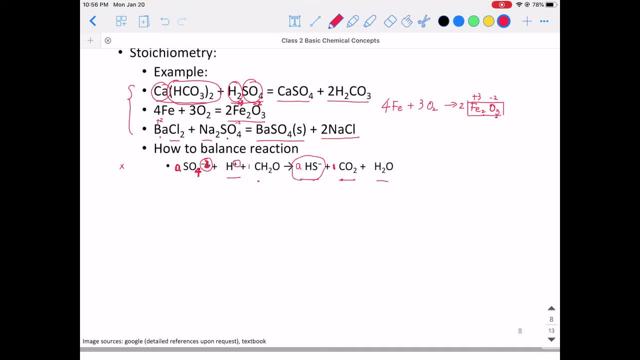 right, But on the right hand side this is only affected by this ion here. So what we can do is we can build up equations. So basically we can assume that the number before the hydrogen ion is b, since we're already assuming that number in front of the carbon, or one here. So let's do a quick balance of both the. 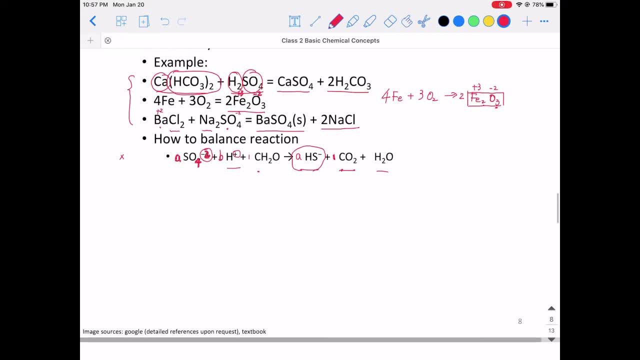 charge and the elements. So on the left hand side we can see that the total charge should be minus 2a, plus b right, And on the right hand side it should be a. So here, please notice that I'm assuming, that I'm assuming. 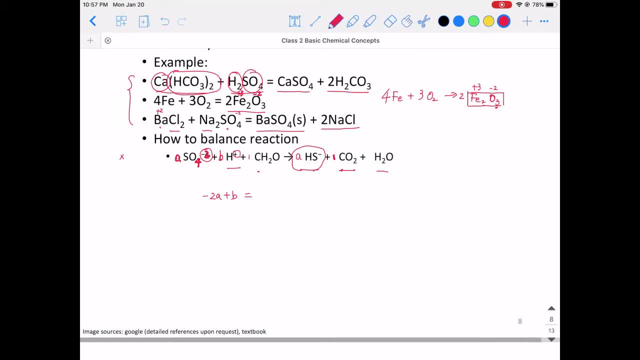 that this is calculating the number of negative charges. So because of that, we need to consider the. on the right hand side, it should be a minus a. So what this means is that the a should be equal to b, right? So now let's make some further modifications here. So a is equal to b. 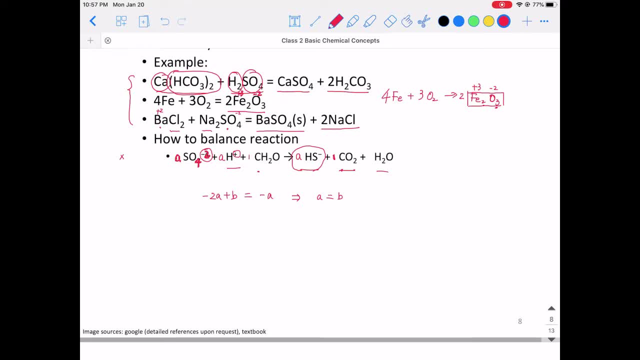 and now we just need to balance. what is the, the number of hydrogen, what is the number of oxygen, right? So then let's build up the relationship for the hydrogen. So let's say, for the first equation, we're trying to build up the balance on the charge, and then let's try to build up the balance of the hydrogen. 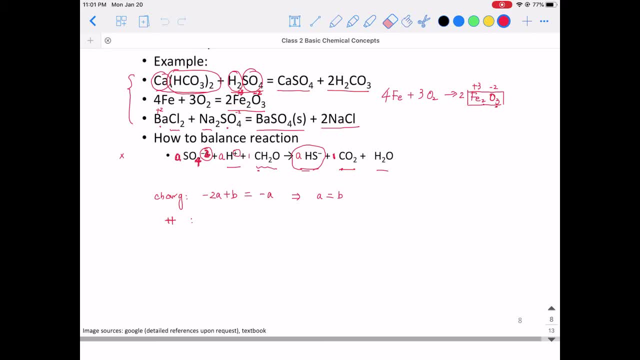 So on the left hand side we need to calculate how many numbers of hydrogen elements are there. So on the left hand side we have a that's coming from the hydrogen ion, and then there are two hydrogen atoms in the formaldehyde compound. that's one multiplied by two. 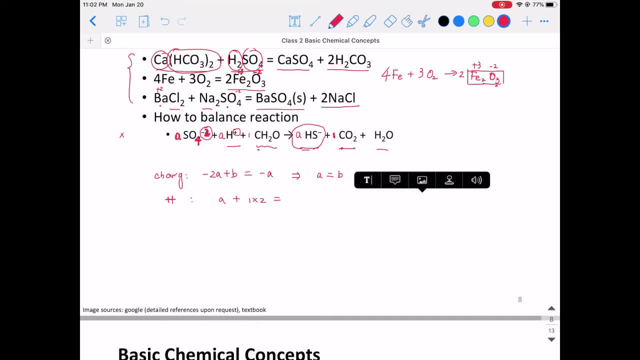 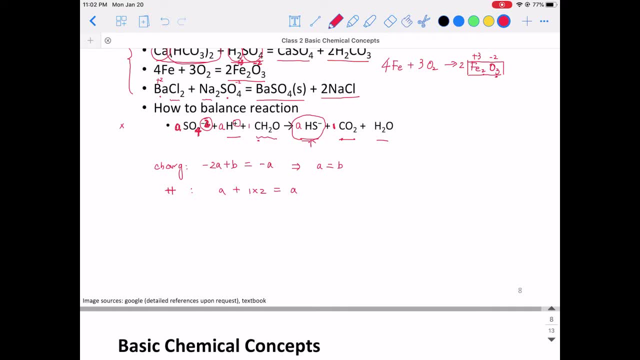 and we're going to look at the number of hydrogen on the right hand side and you can see that this, this compound here, is going to give us or provide us a number of hydrogens, right, And the remaining hydrogens are coming from the water and by building up this relationship, we know that the 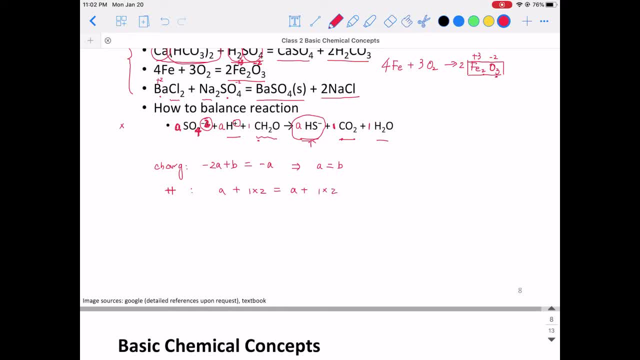 number in front of water should be one, two, right, Because this is going to give us exactly the same number of hydrogen. So we have used up the equation on the hydrogen and then now we need to look at the oxygen here. okay, Let's look at the oxygen and then you can see that for the hydrogen, 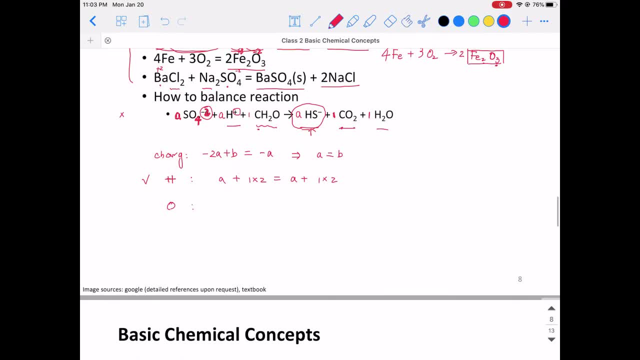 for oxygen. it's getting a little bit more complex because for the sulfide ion it's providing four number of oxygens and we have 4a. then multiply the number of oxygen in the formaldehyde and that should be equal to the number of oxygens on the right hand side and you can see that. 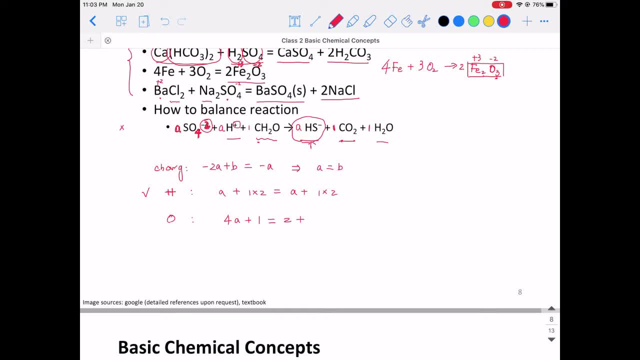 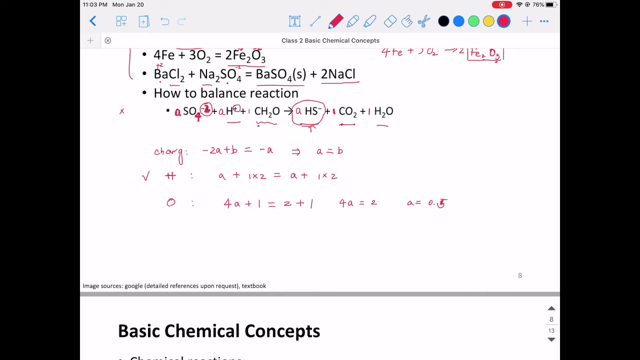 this number is actually two: that's coming from the carbon dioxide and one that's coming from water. okay, So this is going to give us that a or 4a is going to be equal to 2 and a is equal to 0.5, okay, So what this finally means is that if we write out this: 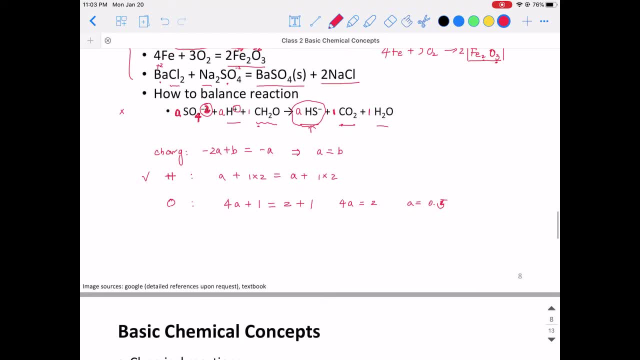 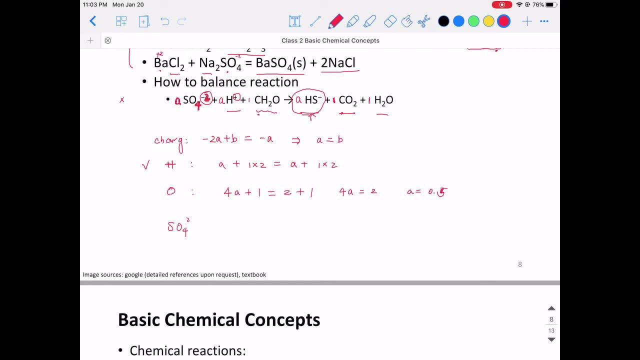 whole equation and multiply by 2 on both hand sides, both the left hand side and right hand side. okay, So that's going to give us the sulfuric acid plus hydrogen ion, plus two moles of formaldehyde. that's going to give us 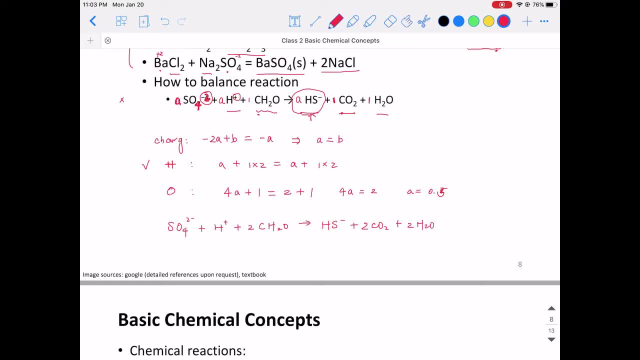 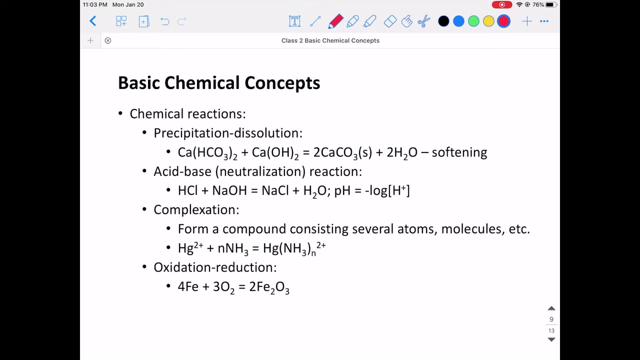 this compound plus two carbon dioxide, plus two water. okay, So this is how we can balance the equation. that doesn't look that very obvious, All right, so now let's look at further concepts, And other than the stoichiometry, which basically balance all of these equations. 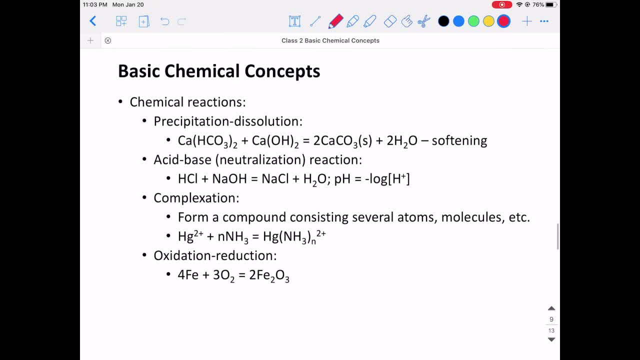 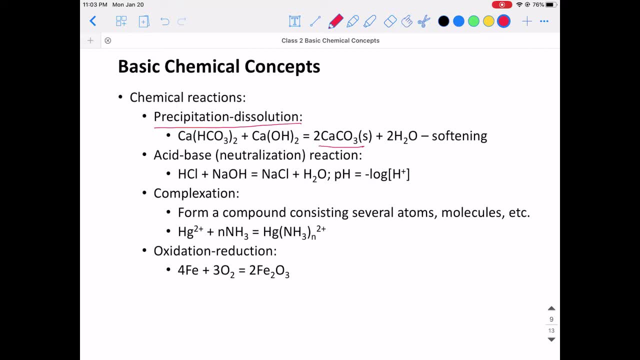 we can also categorize all of these reactions into different types. For example, there are precipitation dissolution equation which is forming us some solids, where these solids can also get a resuspended, or they can further get reacted into ions and further dissolve into the solution. 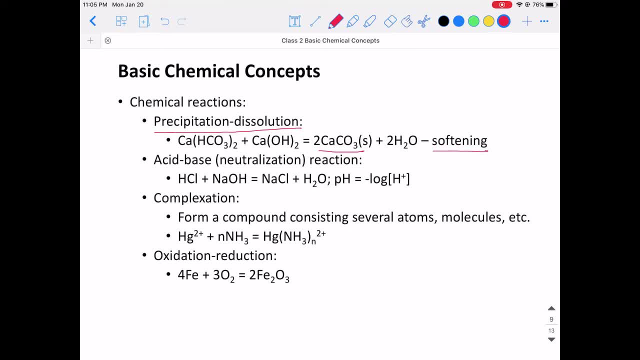 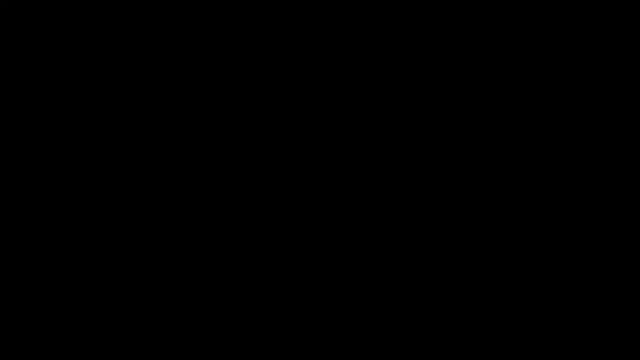 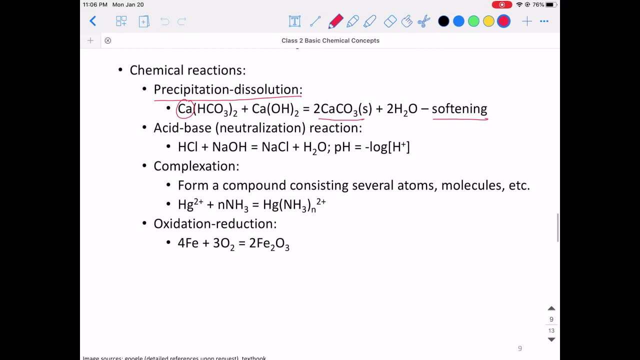 okay. For example, this reaction is typically used for the softening of the water treatment. So basically, we want to remove these metal ions, right? For example calcium or magnesium And so on and so forth. So there are also equations or reactions related with the acid. 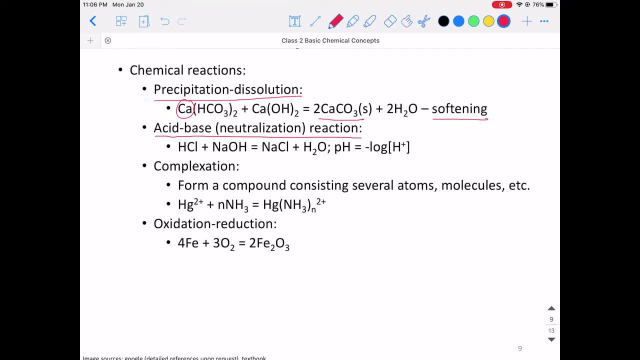 base or neutralization reaction, and we have already given some examples there. So there can be reaction between the hydrogen chloride, which is acid that's reacting with the sodium hydroxide- right, We're going to form sodium chloride- and also water here And further we have the definition. 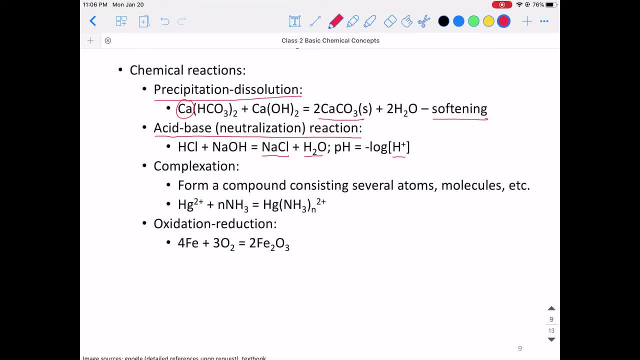 of the pH. So pH is basically the molarity, right? So that is the number of the moles per liter, right? So it's the negative log of the molarity of hydrogen ion. We can further have a look into the definition of the pH later. okay, So there are also some complexation reactions and this is 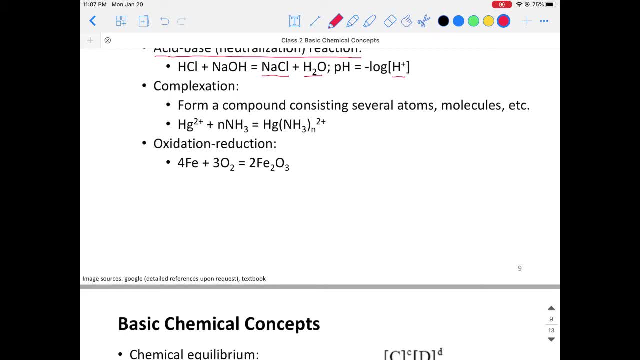 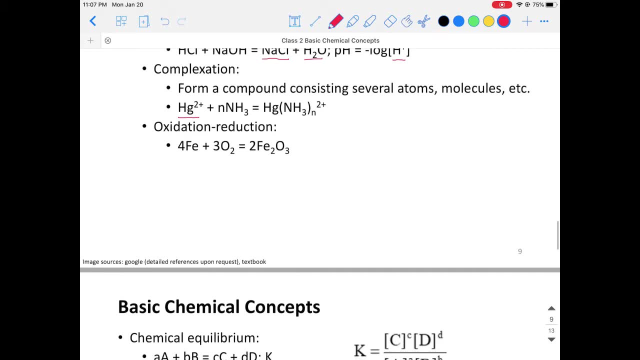 meaning that there are the formation of a compound that's consisting several atoms, molecules, so on. For example, the mercury can react with ammonia and then we're forming these types of complex molecules. because you see that ammonia is really not affected, right? It's not affecting the major structure. 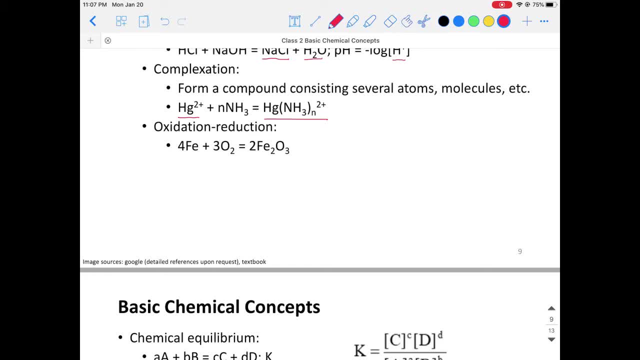 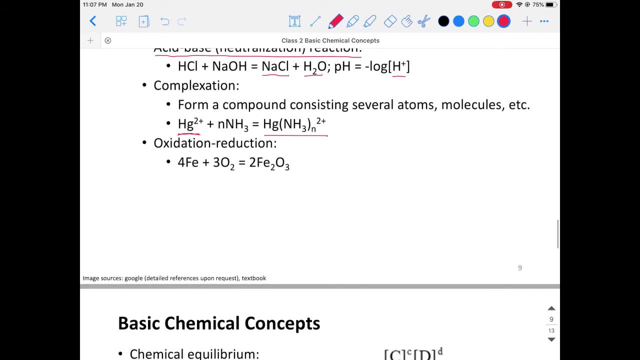 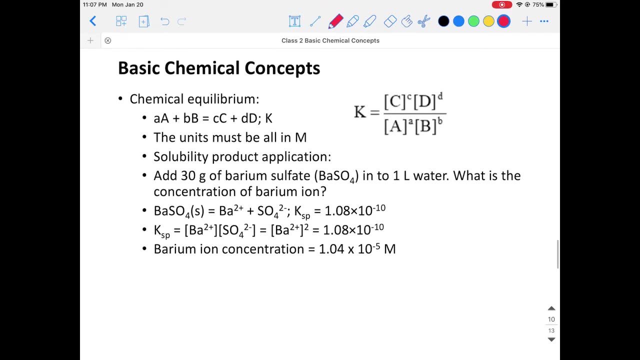 of these compounds here and it's still carrying a charge of plus two, which is coming from the mercury ion here. And of course there is oxidation reduction reactions. For example, we're forming the iron oxide from this reaction here. okay, And further we can go through the concepts regarding 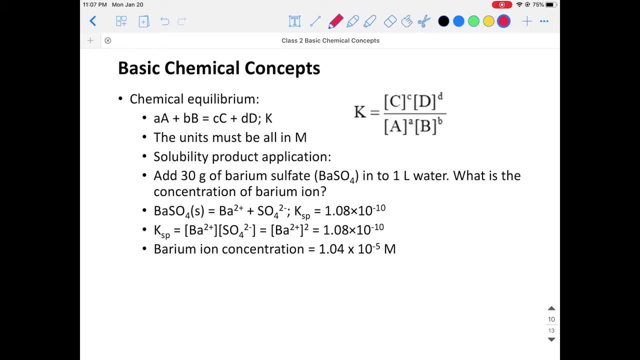 the chemical equilibrium. So the chemical equilibrium basically designates what is the final concentration of all the reactants and products during certain reactions. okay, For example, if we have a reaction that's coming from A number of A species reacting with B number of B species. 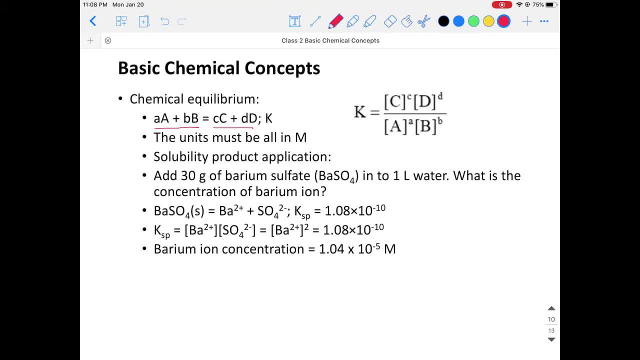 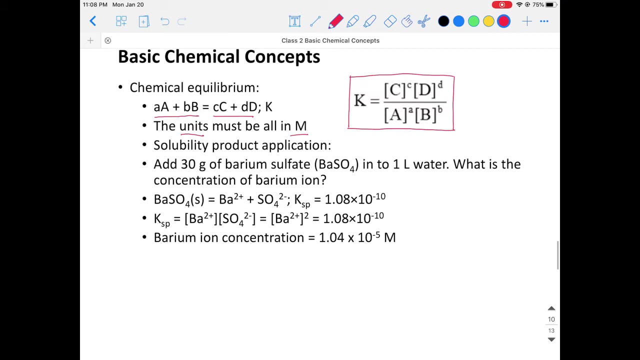 forming C- number of C- and D- number of D. then we can define an equilibrium constant, which is defined in this form. So you can see that there are basically the powers, or the powers of the moles for each of the species. We also need to notice that all of the units must be all in M, which is a molarity here. 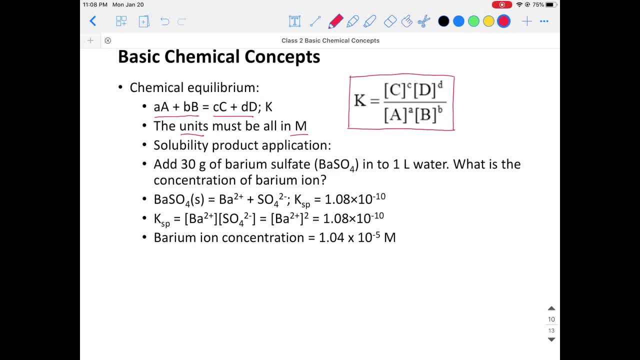 So because if you use different types of units then you're going to get a totally different number of the molecules. So if you use different types of units then you're going to get totally different number of the molecules because you use differences in the equilibrium constants. 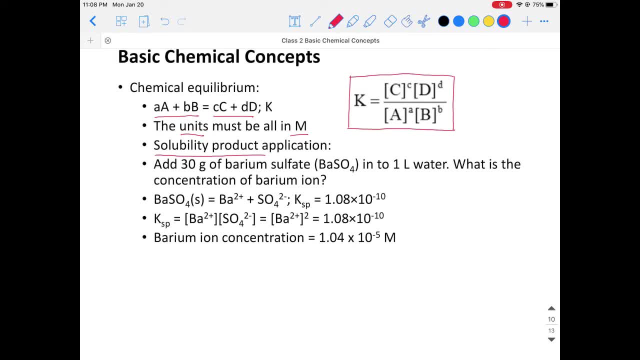 And we can also apply this concept to the solubility. For example, let's say that we're adding 30 grams of barium sulfide, which is a solid, doesn't have a very high solubility. okay, So we're adding this amount of barium sulfide into 1 litre water, So what? 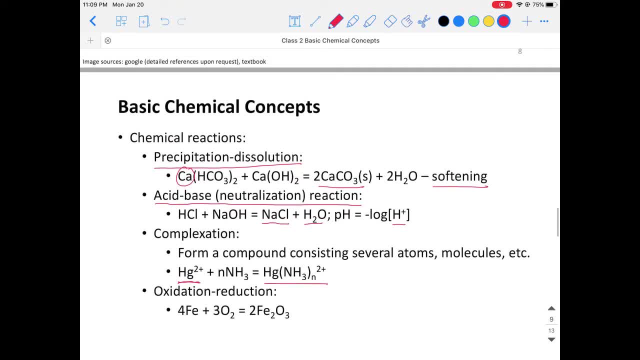 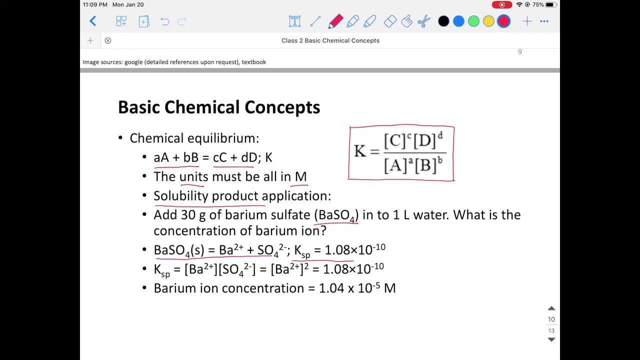 is the concentration of the barium ion. So assume that the dissociation or the sulfate reaction has this type of form and we have a equilibrium constant which is Ksp equal to 1.08, multiplied by 10 to the minus 10. okay, so for these, 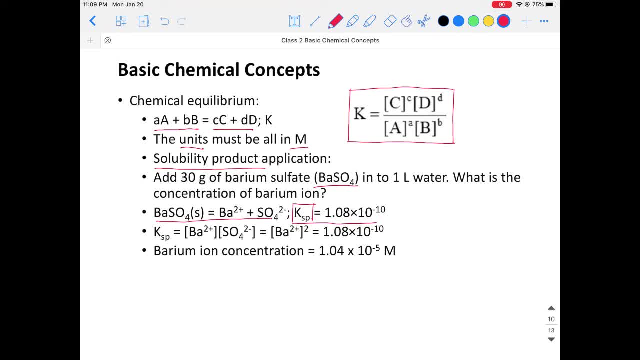 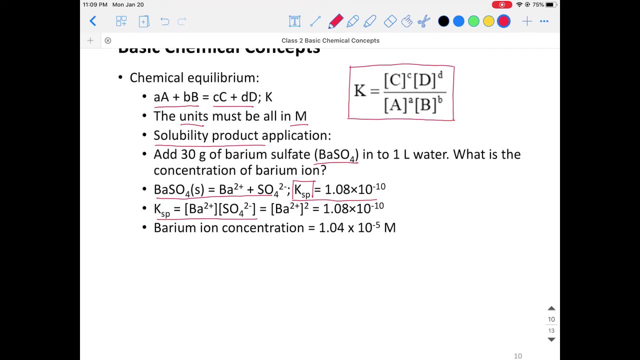 dissolution reactions, the equilibrium constant is just defined as the concentration of the ions, so basically it's the product of all of the ions. so Ksp is defined as the barium ion concentration multiplied by this sulfate ion concentration. We further know that for this type of reaction, if there's one mole of barium ion and 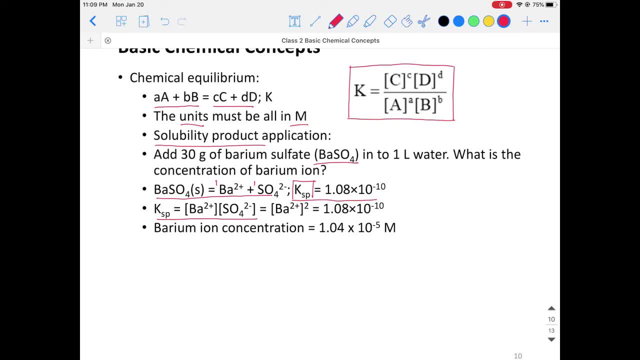 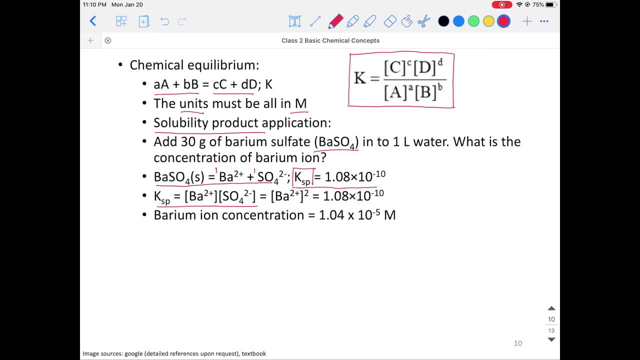 there's going to be one mole of the sulfate ion. because they're all coming from the barium sulfate, the concentration of these two ions should be equal, and so because of that, we're going to have the square of the barium ion concentration equal to this Ksp and further we can basically: 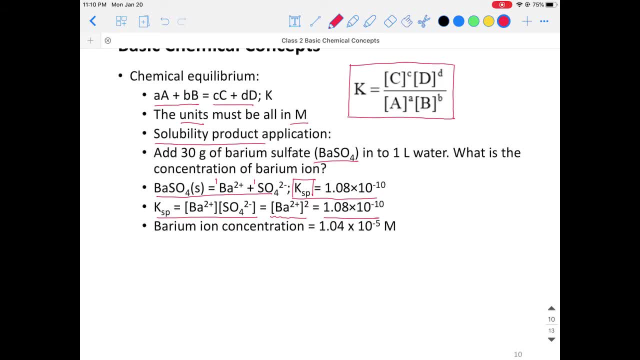 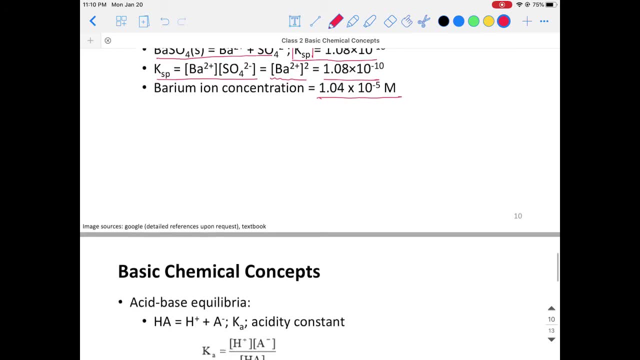 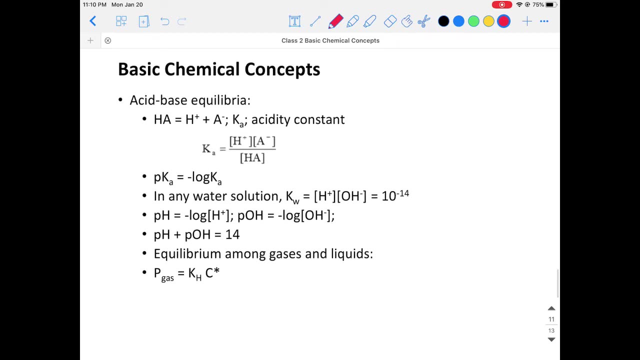 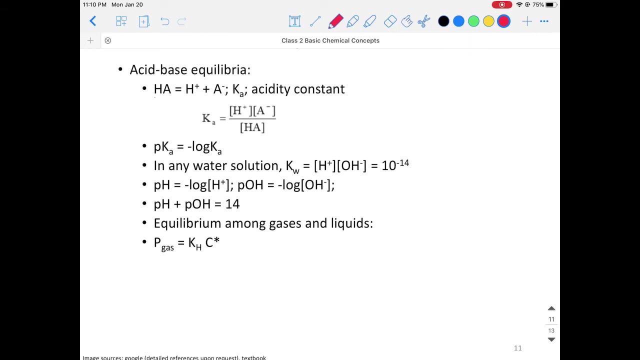 take the square root of this equilibrium constant, and then we can get the concentration of the barium ion or the sulfide ion. And apart from the dissolution equilibrium, there is also equilibrium between the acid and base. For example, for any acid or for any species, they can get disassociated into a. 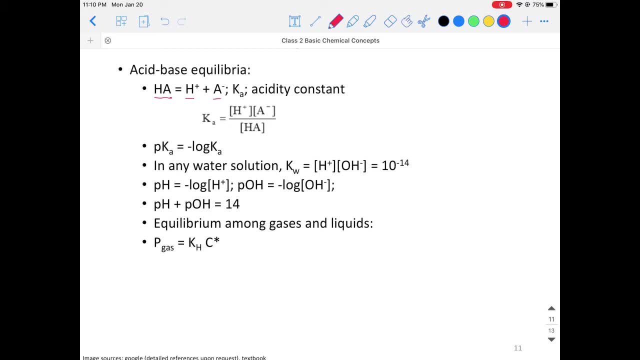 hydrogen ion and also to a negative ion. So we define this Ka as the acidity constant which can be written in this form. And further we can define a pKa, which is a negative log of the Ka. So we can apply this concept into water, For example. water is going to have. we can consider: 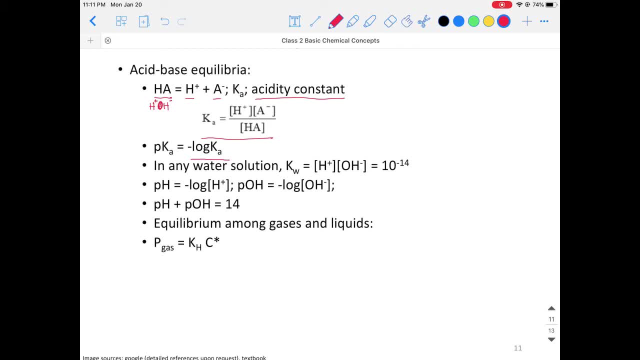 water as hydrogen, with the hydroxide ion. So we can assume that there is a disassociation between the, the water, between these two types of these two ions, and then we're going to define a Kw, which is- we can see that- as the acidity constant of water. 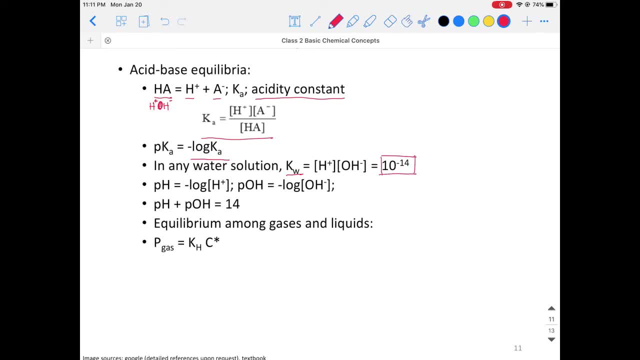 So you can see that this constant have a single or constant value of 10 to the negative 14.. Further, we can define the concept of pH, which is a negative log of the hydrogen ion, And we can also similarly define a concept of pOH, which is a negative log value of the hydroxide ion. 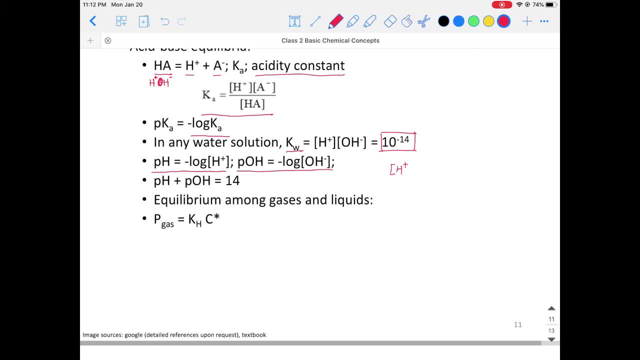 So let's say, for example, if we take this reaction here, equal to 10, to the minus 14, and if we take log on both sides, what's going to happen? We're going to have log of hydrogen ion, hydroxide ion, hydrogen ion, hydroxide ion, hydrogen ion. 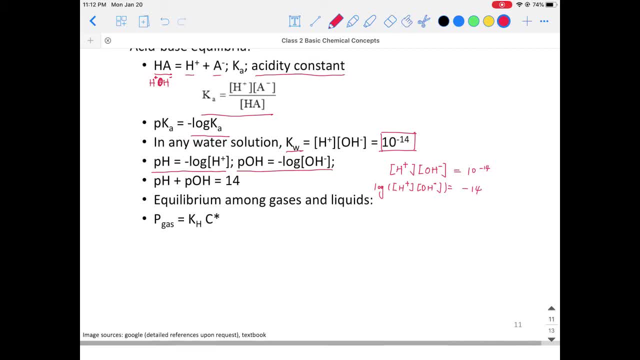 i equal to minus 14, right and further. we know that for log it has the property of, so the product, or the log of a product is going to be the is going to be a, it's going to be the sum of two logs. it's negative 14 and if we further move the negative sign, 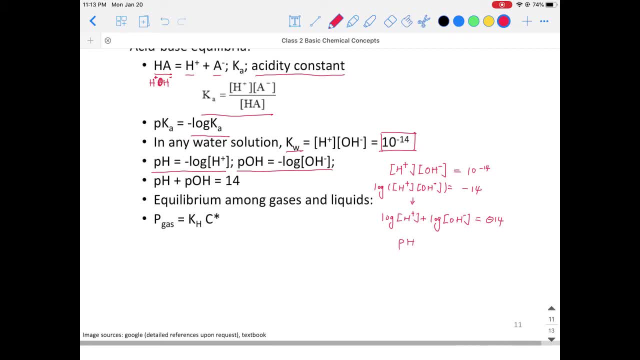 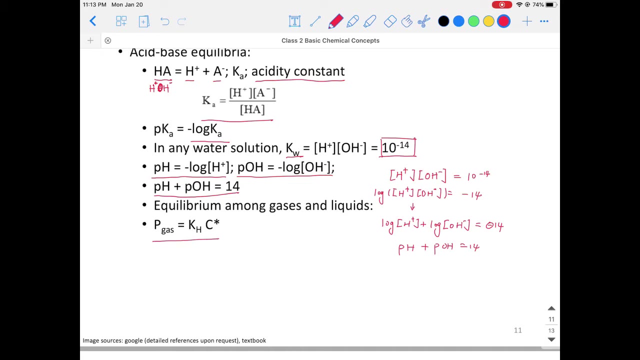 on to the left hand side. okay, so that's going to give. basically give us pH plus pOH equal to 14, which is the relationship goes around here. okay, so we can also have the equilibrium among gases and liquids, and this is called the Henry's gas law. so basically the 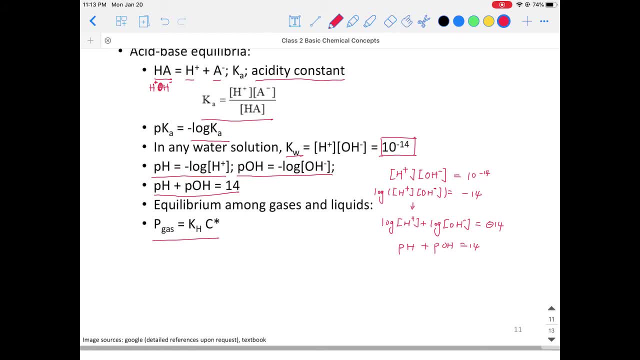 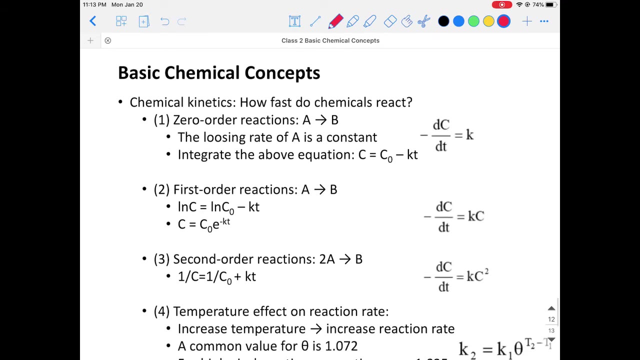 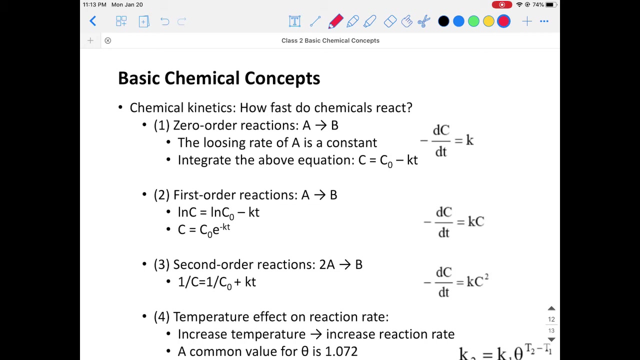 vapor pressure of certain gas. that's going to be proportional to the concentration of the species in the liquid. okay, so we call this constant as the hundredth constant, and this applies for the dilute solution. so we learned about the equilibrium of the reactions. so equilibrium is not only the parameter that's describing a reaction. 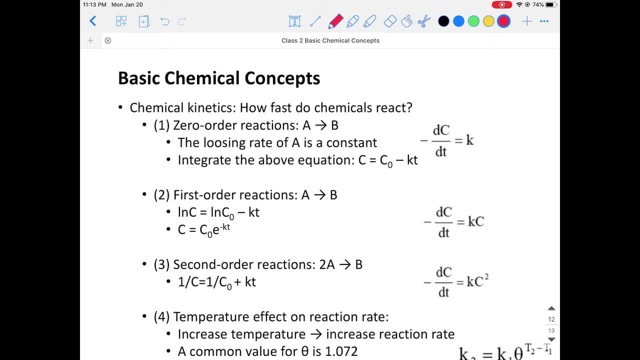 because Voldenberg-R******* does so at least sometimes. we just want to get bees to act- decides what is the final concentration of all of the products and the reactants. but how fast or how fast do these concentrations reach the final concentration? and this is decided by the chemical kinetics. So for all of 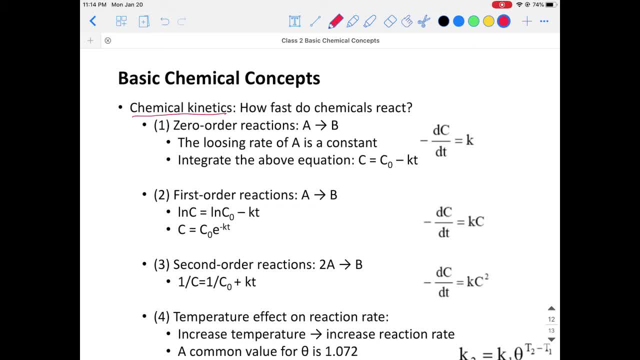 different types of the reactions. we can define them into different orders. They can be a zero-order reaction. for example, let's say that the species A is converting into species B. The zero order means that the losing rate of A is a constant. So if we write that out in the form of a differential equation, then the 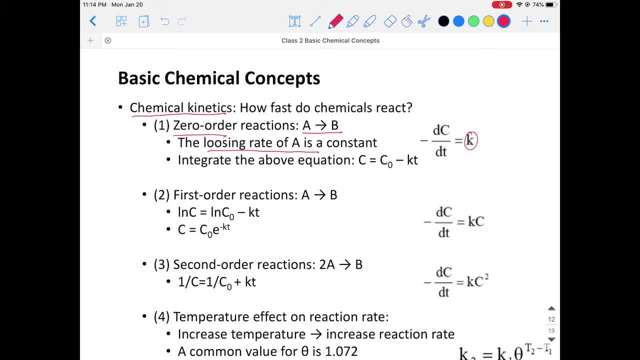 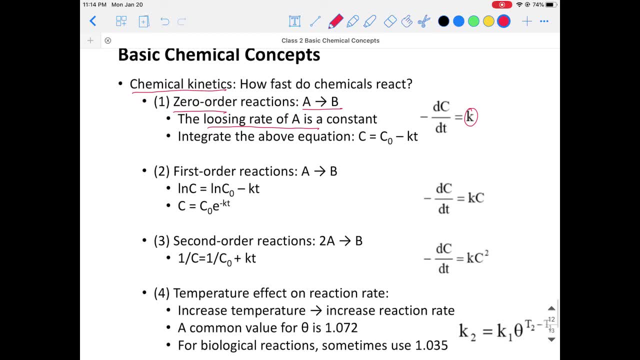 concentration of A or the decrease of the concentration of A is going to be a constant k here And because of that, if we do an integration of this equation, we're going to have a constant k. So, for example, if we do an integration of this equation, we're going to have a. 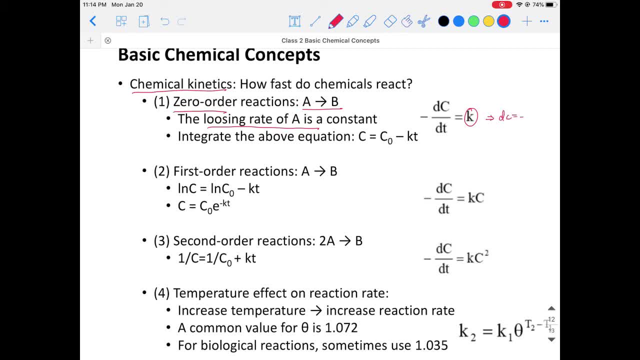 the concentration is going to be equal. so basically you have dC equal to negative k dT. So C is going to be a constant C0 multiplied by kT and this is going to give us the concentration for the C here. But we also need to 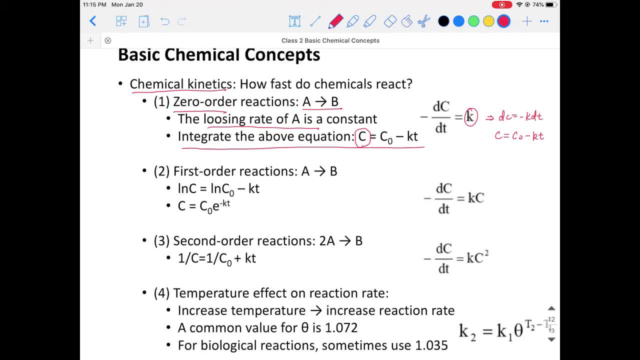 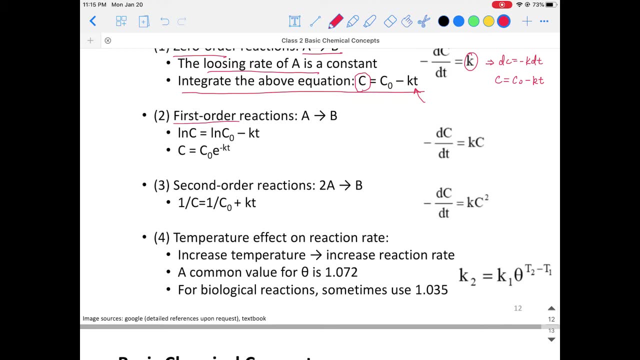 notice that the C or the concentration of the species A cannot be negative, right? So there is always a range of time, A range of time that works for describing the concentration of the A species. So there are also first-order reactions and most of the reactions. 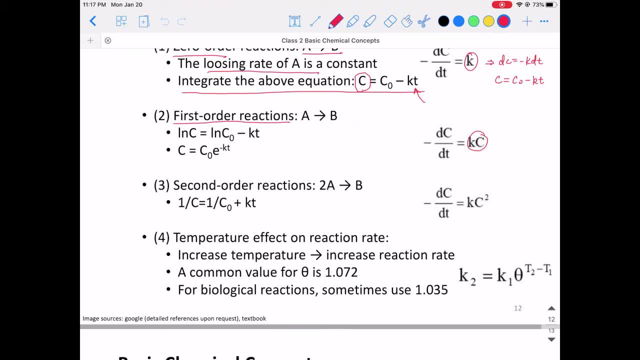 that's happening naturally from the industry are first-order reactions. They will follow this type of rule here. And how do we solve for the concentration of A if it follows the first-order reactions? And what we can do is that we can rearrange this differential equation. Let's say we have dC divided by C equal. 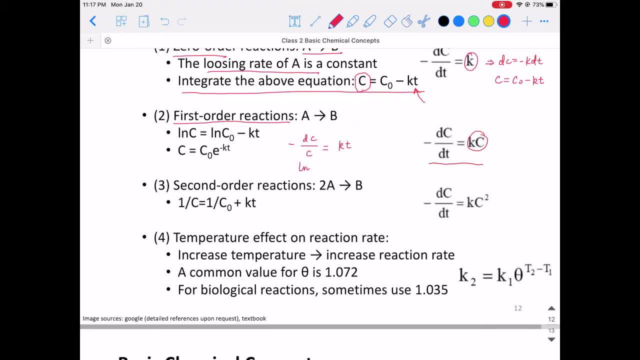 to kT. okay, And further, if we integrate on both sides, we know that we're going to get a log C here on the left-hand side. We're also going to carry this negative sign here. It's going to be kT. You should also notice that. 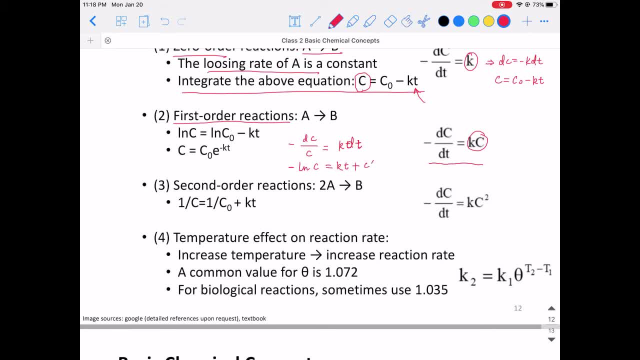 here it should be kdT, okay, Plus a constant. Let's assume that this is C prime, okay, So further we can rearrange this and as it's going to give us basically C, it's going to be equal to exponential of negative kT plus C prime, okay. 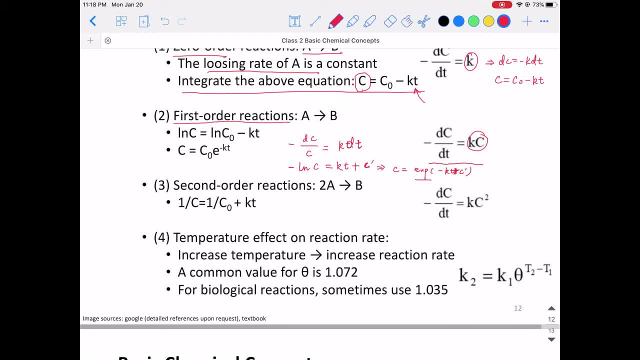 And we know that for the exponential calculations here the exponential of two terms adding up together, we can separate that into exponential of negative C prime multiplied by exponential of negative kT And then we can assume this term as C zero, negative kT. okay, You need to notice that here. the sign here should be negative kT. okay. 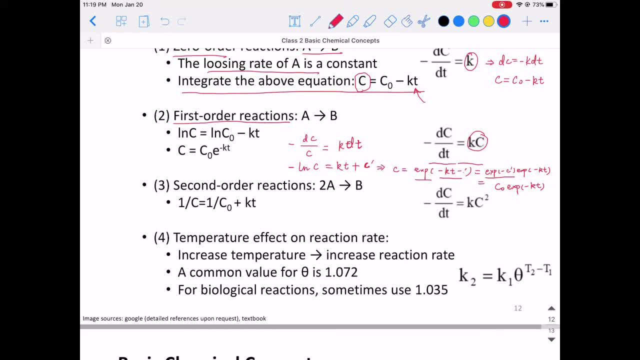 And then we can assume this term as C zero, negative kT. okay, You need to notice that here. the sign here should be negative kT. okay, You need to notice that here. the sign here should be negative c prime. all right. 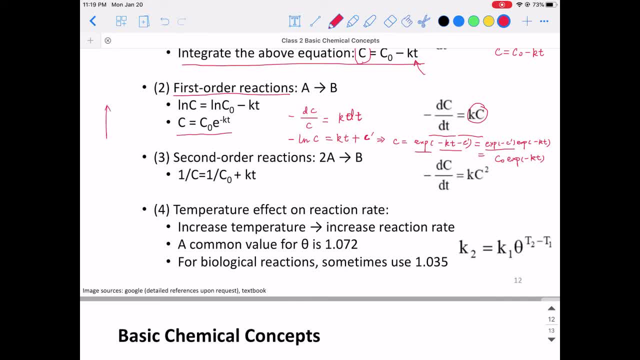 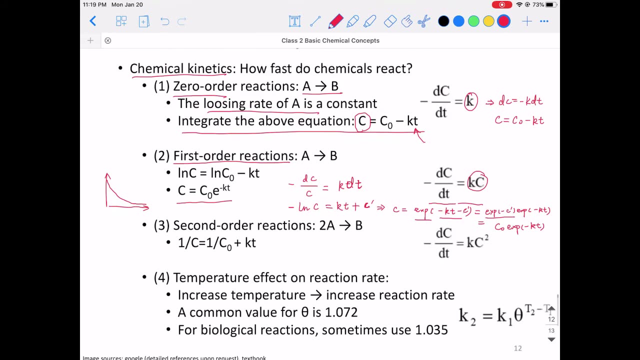 So this is how we can obtain the concentration of C as a function of time, And if we further plot it out, you can see that this is a monotonic decrease of the concentration and this follows the rule of exponential decrease. And similarly we can these reactions. they can also follow second-order reaction. 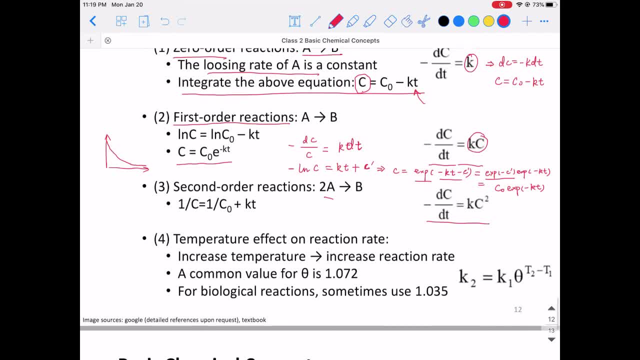 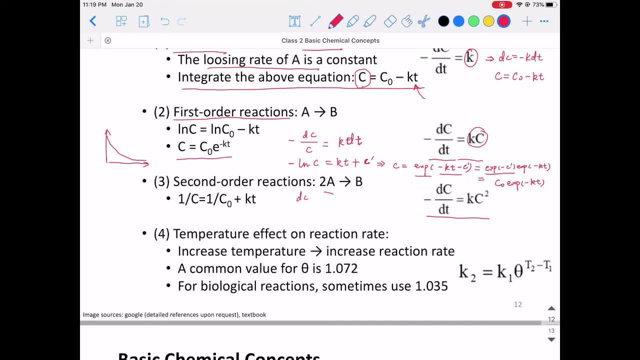 What second-order reaction is that the decrease or the reaction rate of the species A is going to be a constant multiplied by the square of the concentration, And we can also do some rearrangements of this differential equation and that's going to give us kT. 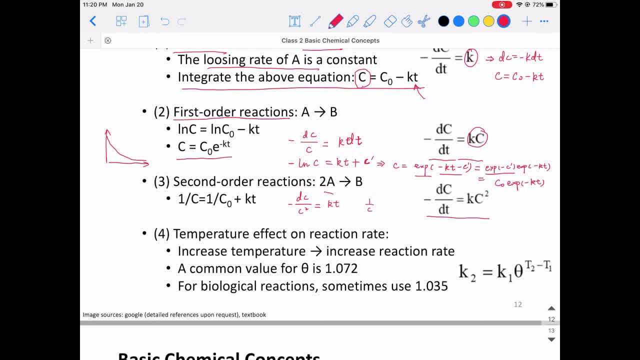 right, And if we do an integration on both sides, then we're going to have 1 over C plus certain constant right. It's equal to kT and this is going to be the. And if we do an integration on both sides, then we're going to have 1 over C plus certain constant right. It's equal to kT and this is going to give us kT and this is going to be the. 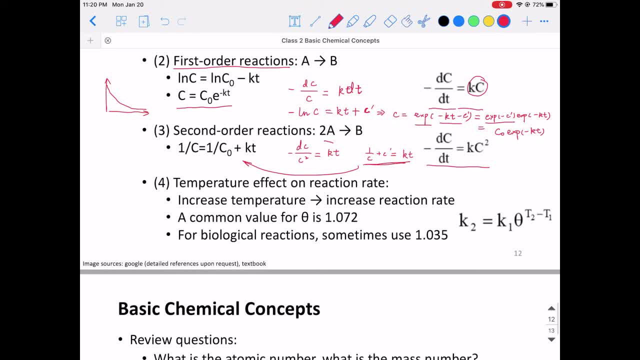 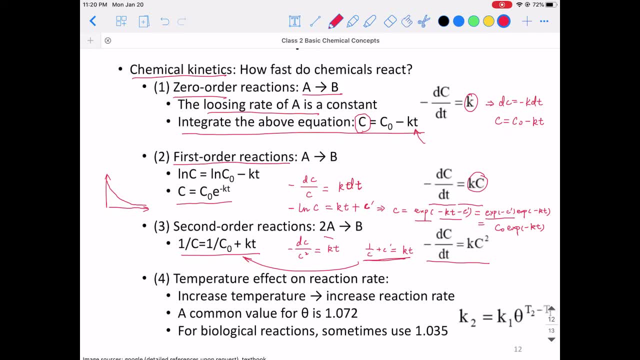 how we can obtain the relationship here. So this is going to be the final concentration as a function of time. all right, So this describes the reaction rate, or how we can calculate the concentration of the reactants if they are following either 0th order, 1st order, 2nd order reactions. 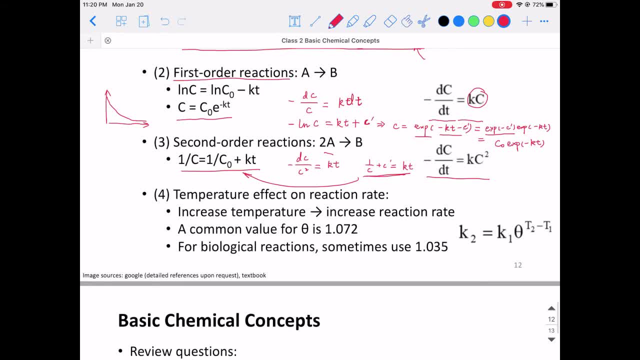 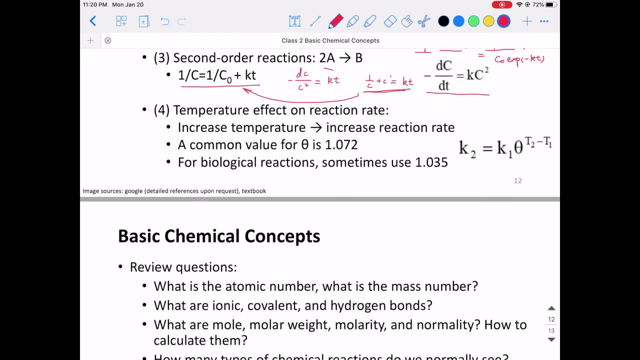 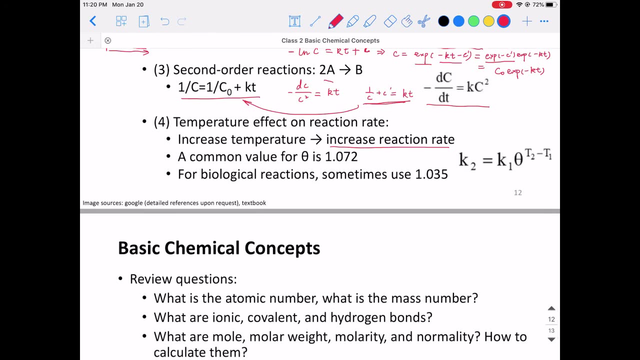 But we haven't discussed anything about the k here. So it turns out that k is a strong function of temperature. So what happens is that if the temperature increases, the k number is also going to increase, and it's going to cause an increase of the reaction rate. 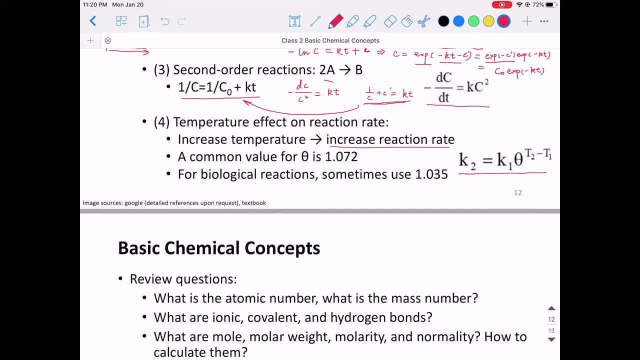 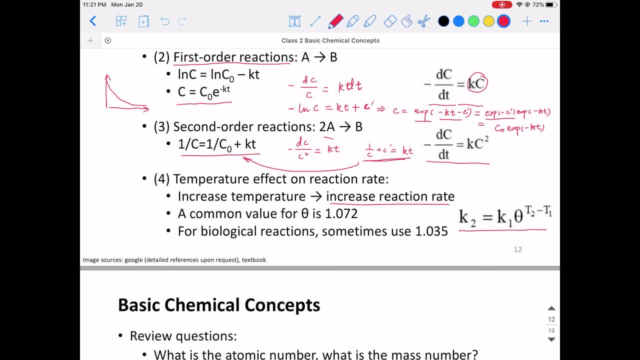 And typically in environmental engineering we use this equation to describe the temperature dependence of the rate constant here. So we call this k as the rate constant And you can also find out that if the theta or if k1 is obtained under T1,. 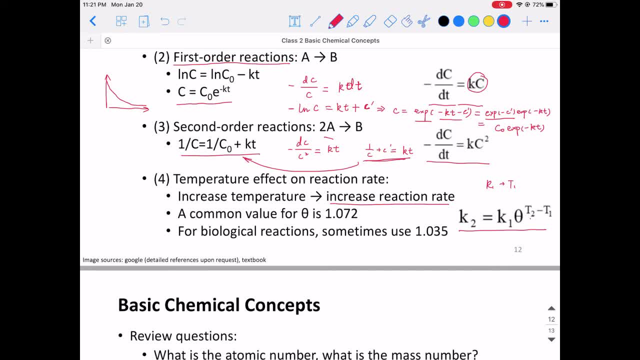 then if the T2 is larger than T1, then the k2 is going to be k1 multiplied by this term here. okay, And since theta is a positive number, so say theta is a number that's larger than 1, then this means that if T2 is larger than T1, we're going to have k2 larger than k1, simply because this term is larger than 1, okay. 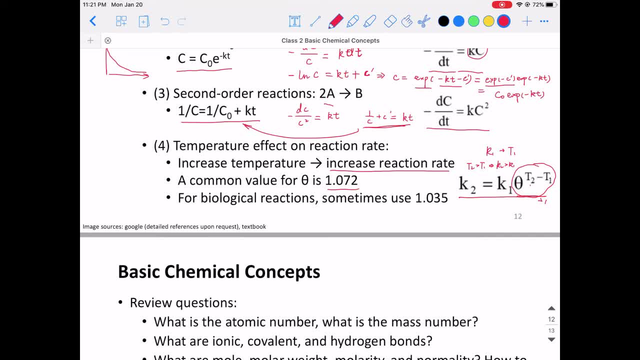 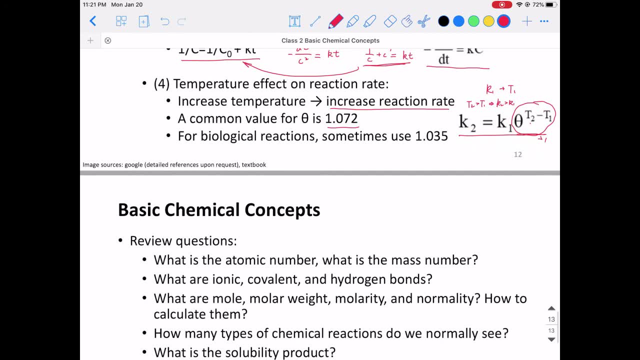 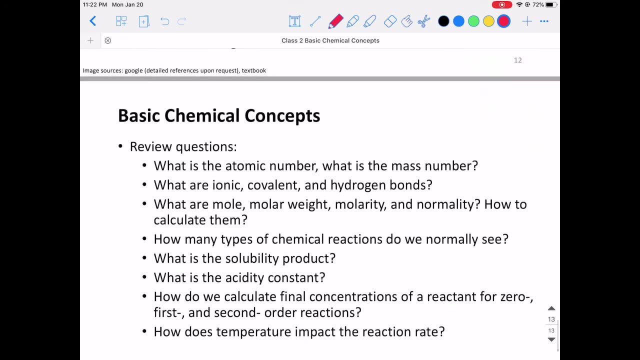 And in environmental engineering typically we use this equation to describe the temperature dependence of the rate constant. So we use the value of theta equal to 1.072 to calculate the rate constant under different temperatures And also for biological reactions. sometimes we'll use a value of 1.035 to determine the rate constants, okay. 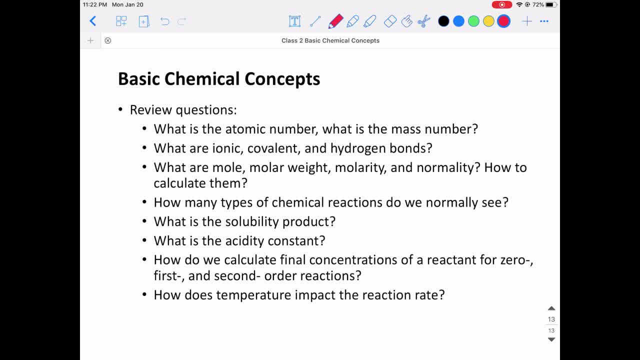 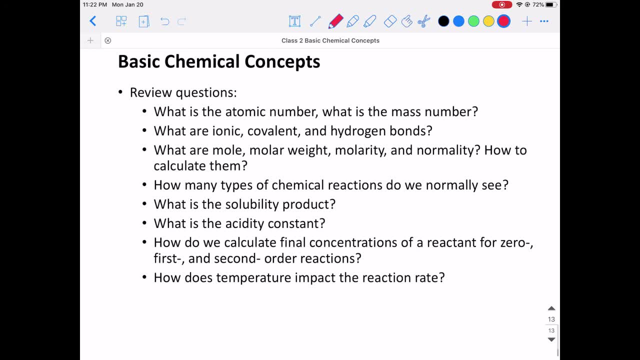 So, finally, you can see that there are really indeed a lot of basic concepts that we use in environmental engineering, and we want to quickly review all of these concepts here. okay, So we have to know what is the atomic number. So atomic number is the number of protons, right? 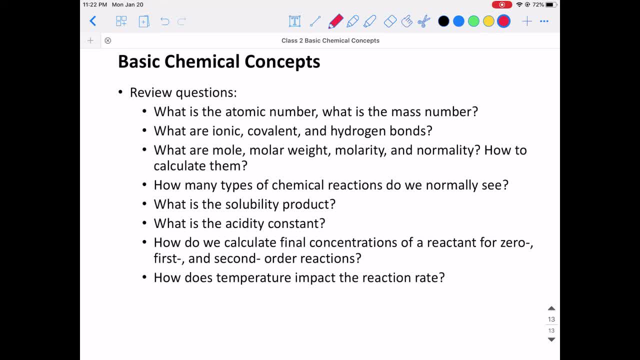 What is the mass number? It's the sum of protons and neutrons. So also what is ionic, or what are ionic, covalent and hydrogen bonds? So you can see that some of them are because of the chemistry, some of them because of the physics. okay,